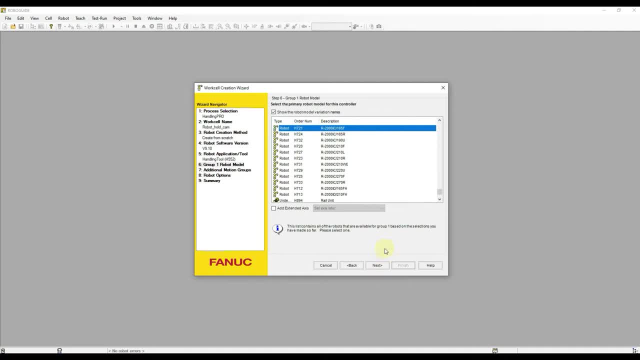 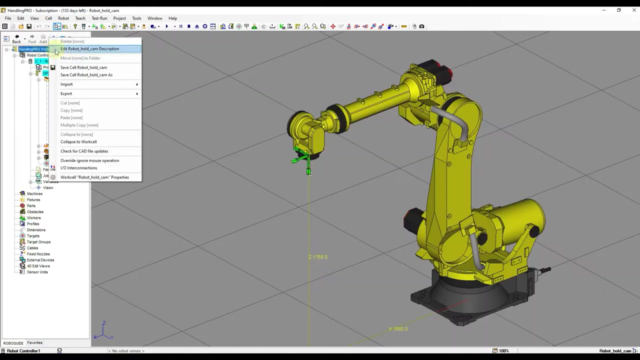 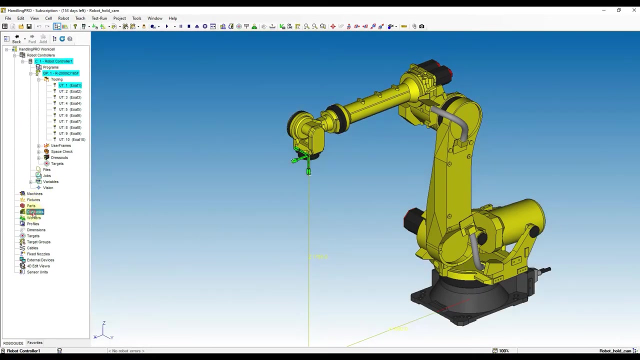 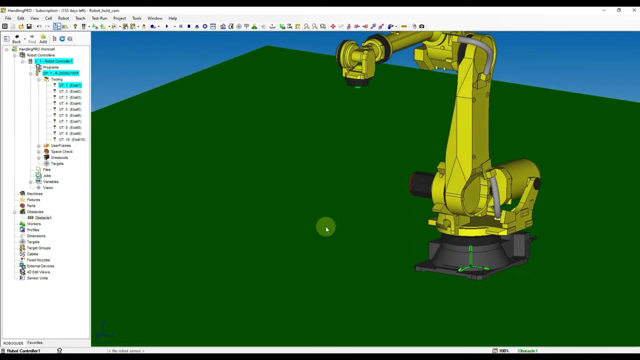 Use the default selection robot to continue the creation wizard. Search irVision and then select the irVision2d package and irVision2dv. Prepare the work cell accordingly. Now add the base plate for our robot. Now add the base plate for our robot. 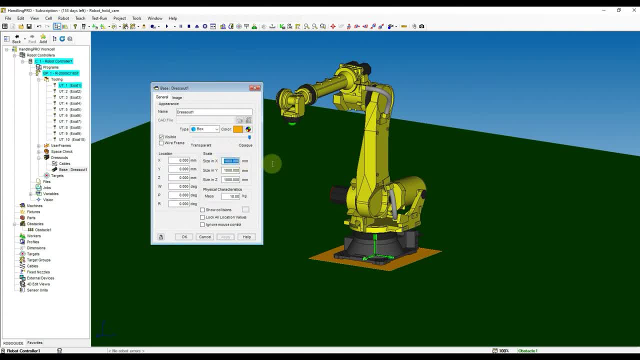 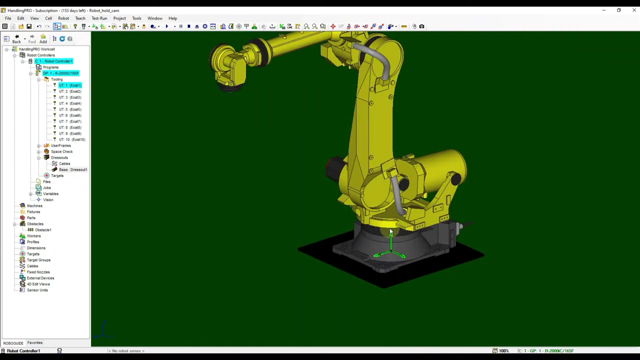 Hold ALT as the base plate and click OK to close it. Remember to change robot height according to BasePlateThickness. We need to reserve some space for the camera to mount on RoboEnd of effector, So select the robot end of effector to add in a more visible reflection. 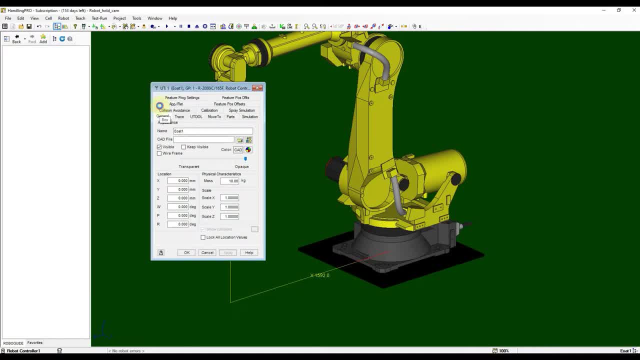 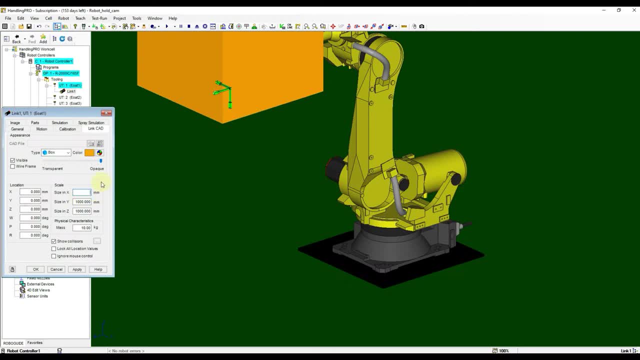 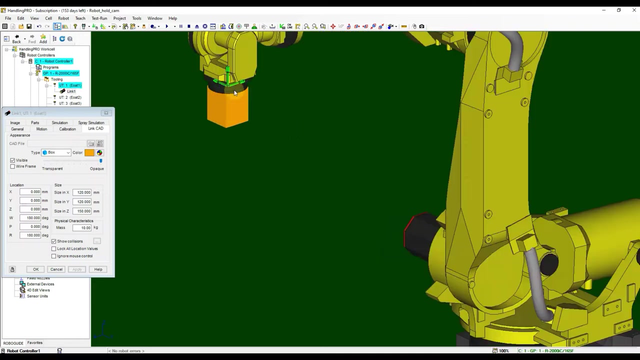 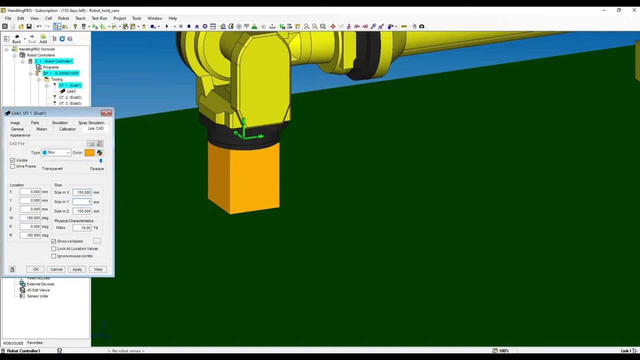 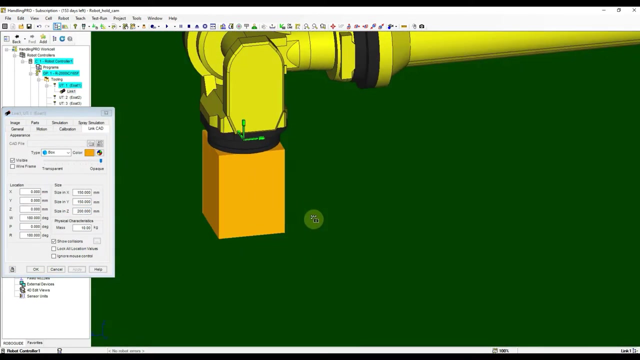 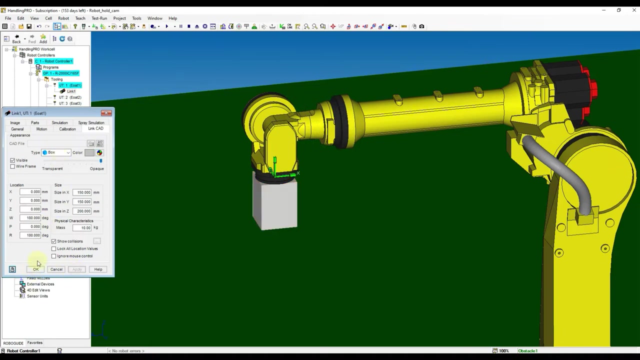 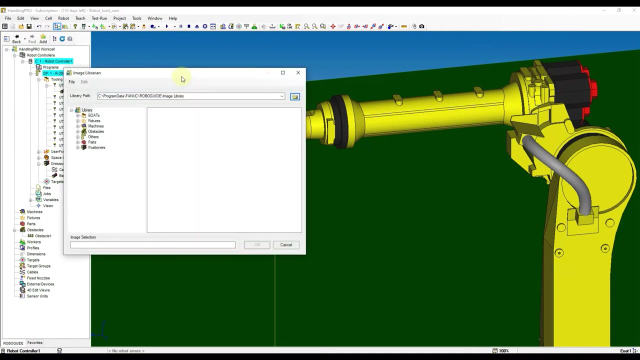 select Add link from the UT1 and then select Box. After that set the size and location, Tune the size of box slightly bigger than the flange, Add link at UT1 again and then select CAD Library From the menu list. select Pointer. 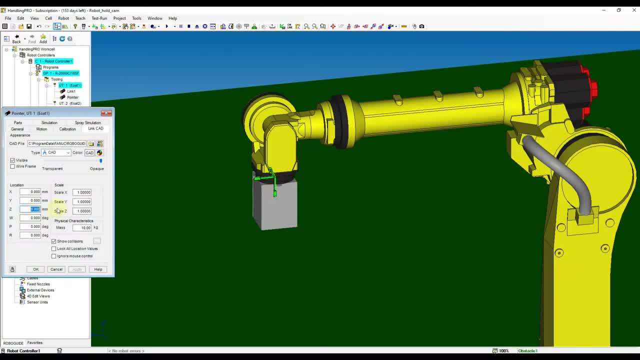 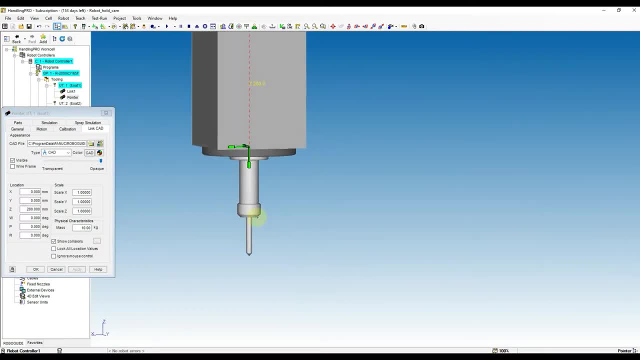 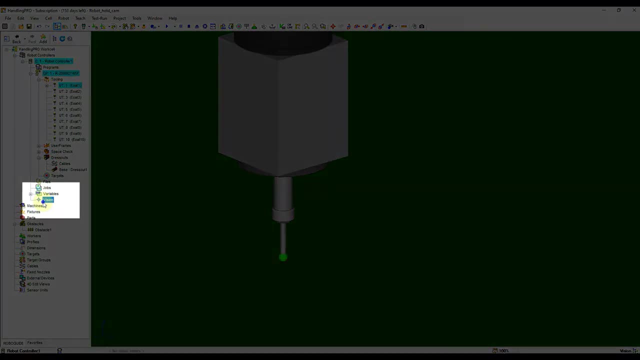 Change the location of the pointer CAD to attach at UT1.. Let's add another location to the Pointer CAD and then select Add. After that, set the size and location of the flange at the end of the box. Now enable the Vision Simulation from the Vision menu at the Cell Browser. 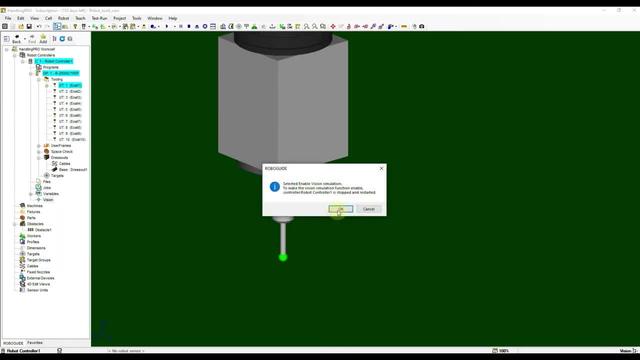 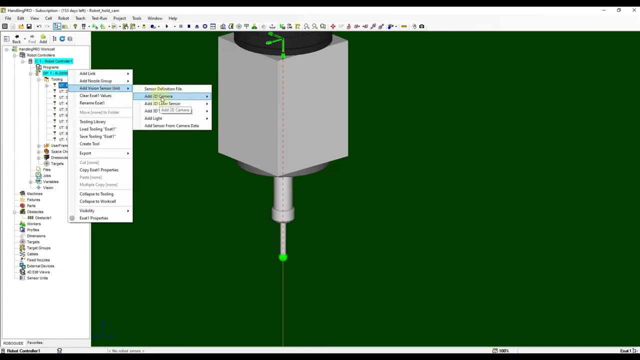 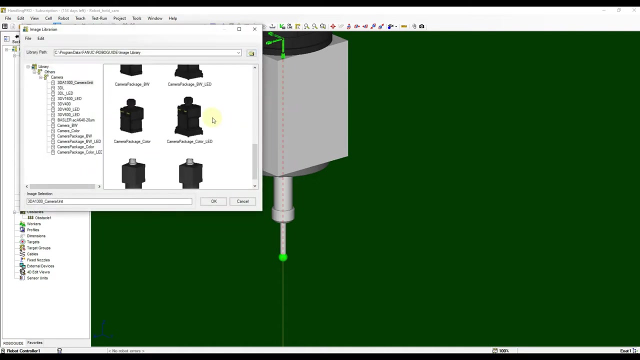 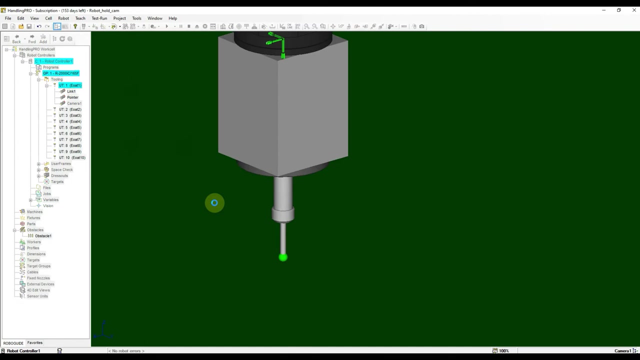 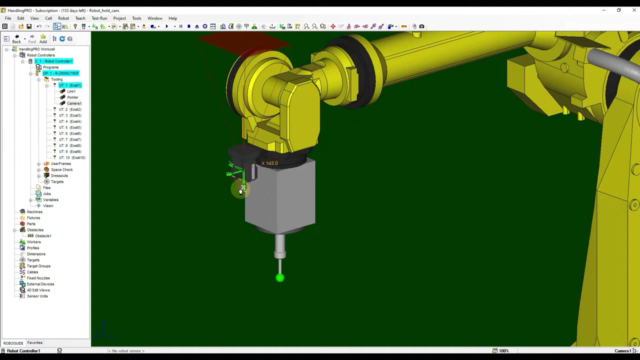 Right-click to change the properties. After controller rebooted, go to UT1 again and right-click Select Add Vision Sensor Unit option and then Add 2D Camera and then CAD Library. Select the same camera. Move the camera CAD to correct orientation with the triad. 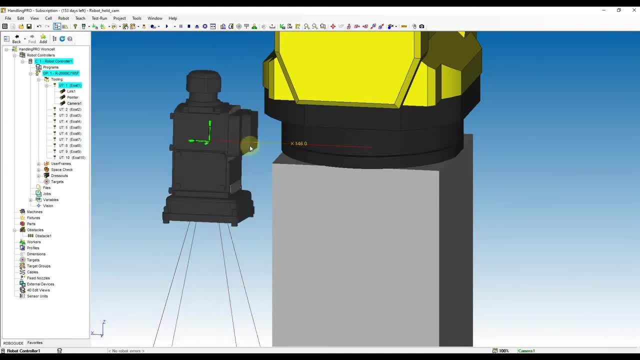 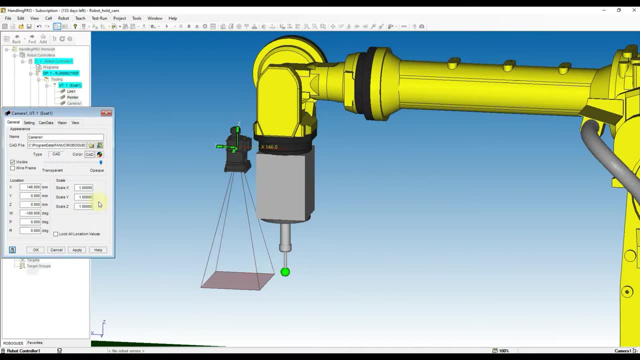 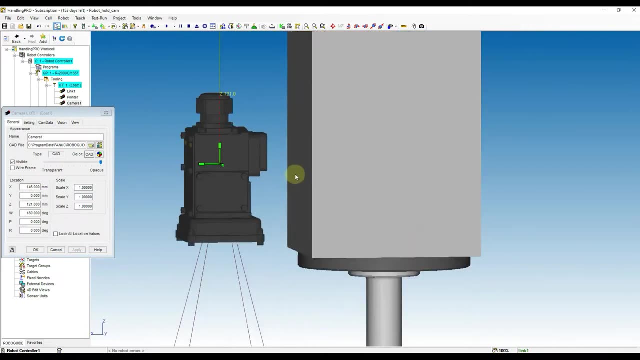 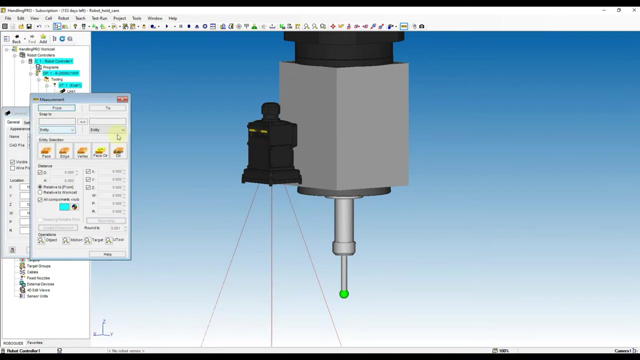 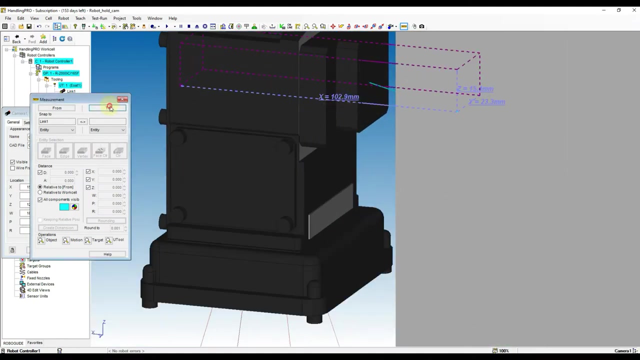 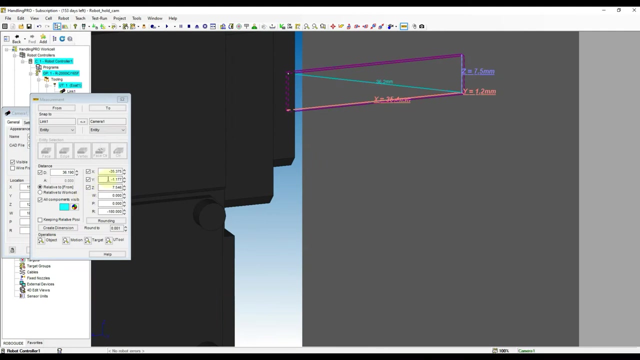 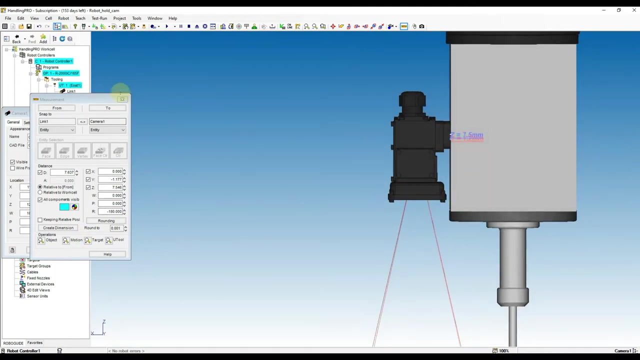 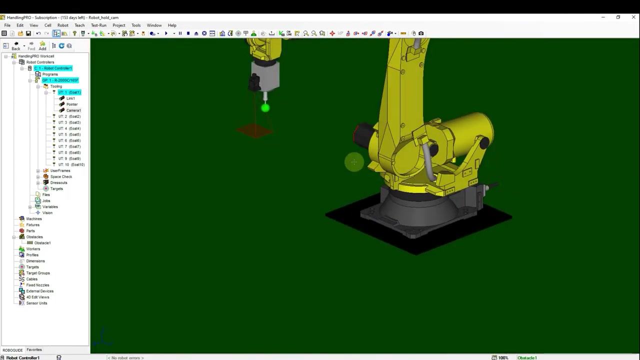 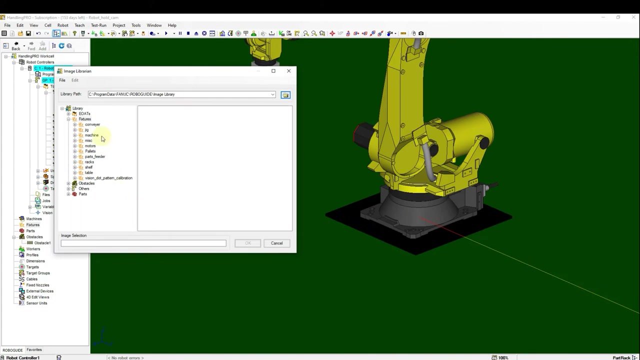 Round off the imperfect values and then move the camera to near to the position we want. Use the measurement tool to move the camera to attach to the EOAT link. Add fixture to the work cell with the Fixture menu at the Cell Browser. From the CAD Library menu, select Table menu and then select the table accordingly. 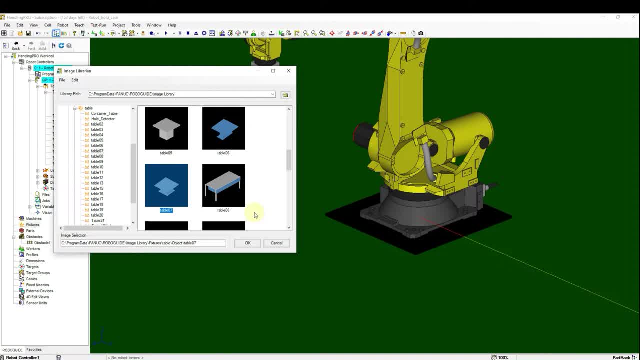 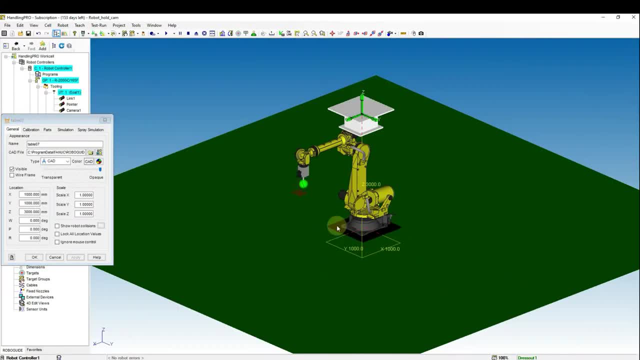 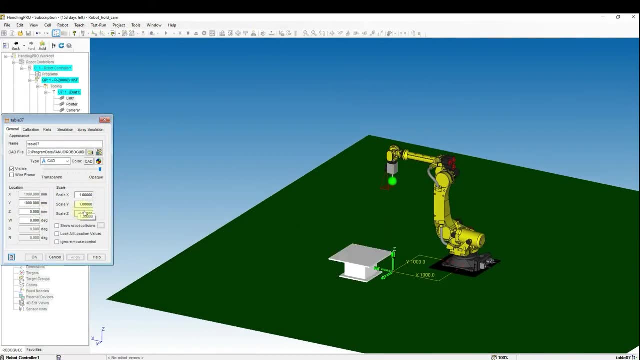 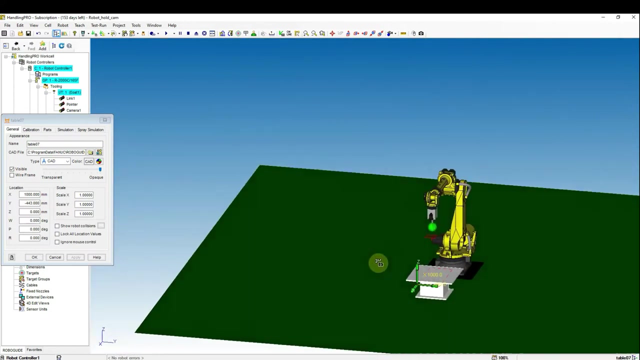 According tolied, you can adjust theoolity value of the tab, Change the table location and size. now Take a look and see if all keys are selected. You will also see the various folders under the categories. The size of the table was adjusted as at the beginning. 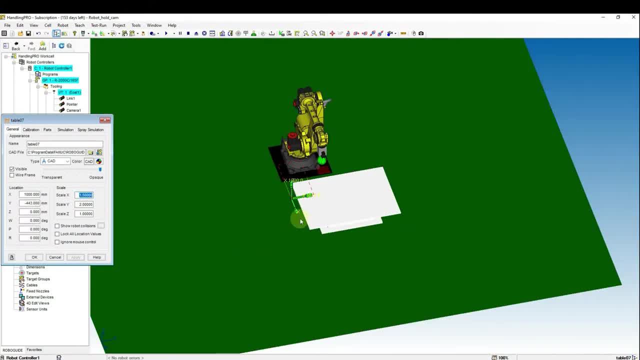 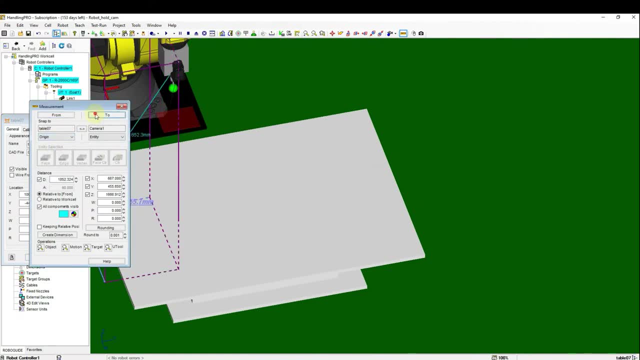 Enter the information for the configuration page on the part Show the location Open the 1950 USB Porter wants was setting with the scale value. We have to measure the table actual size ourself so that the location of table center can put nicely at the covered range of the robot working. 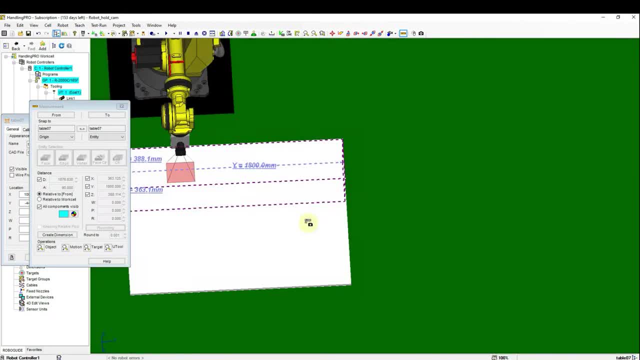 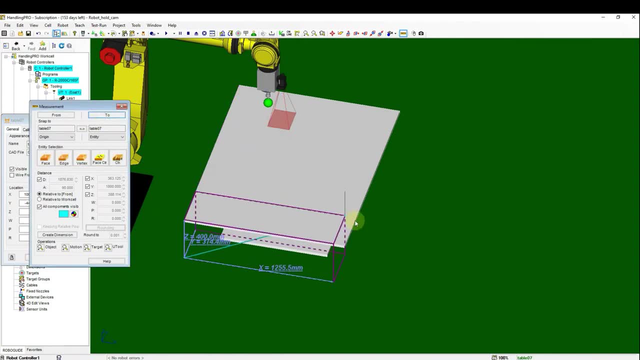 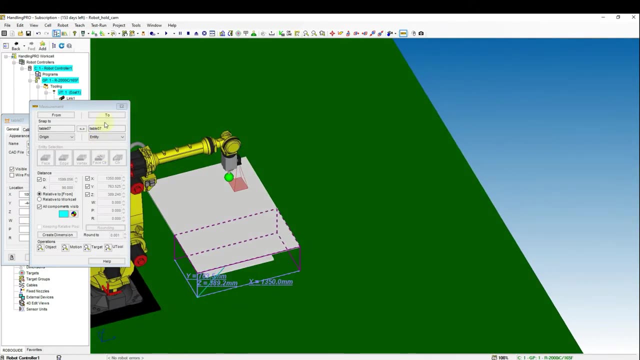 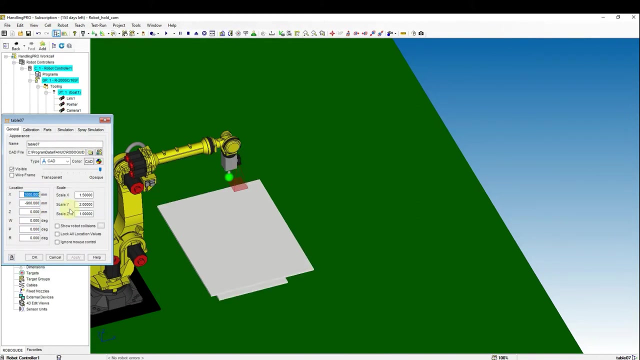 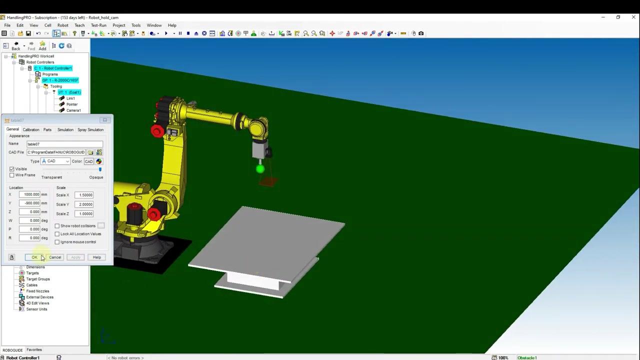 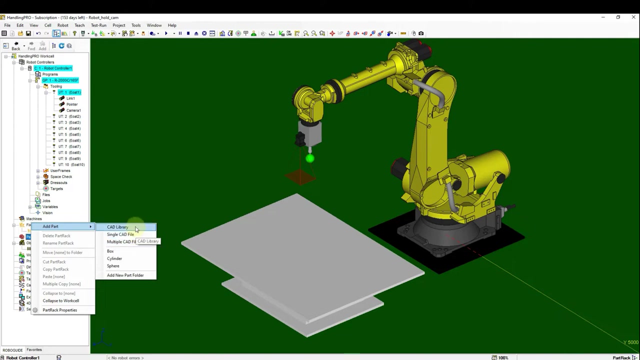 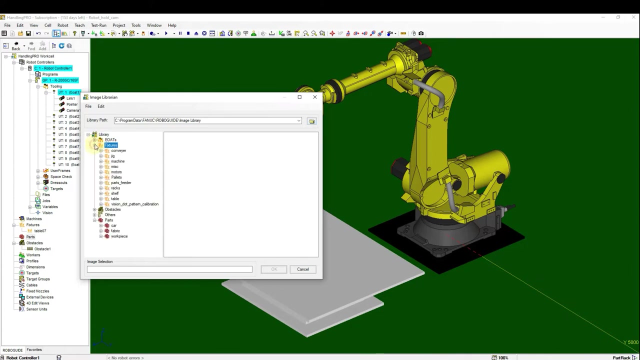 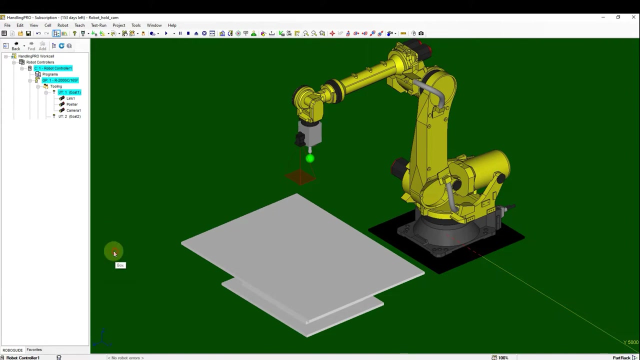 zone. Now set the location coordinates of table to center of robot. Add the calibration jig S part to the table and then locate it to the top surface of table. Add another part to the work cell with box. Then change the name to glass panel. 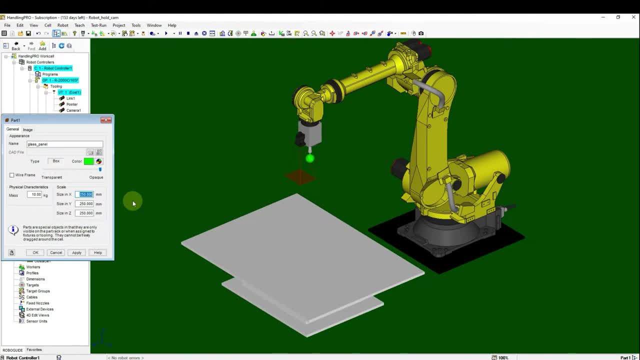 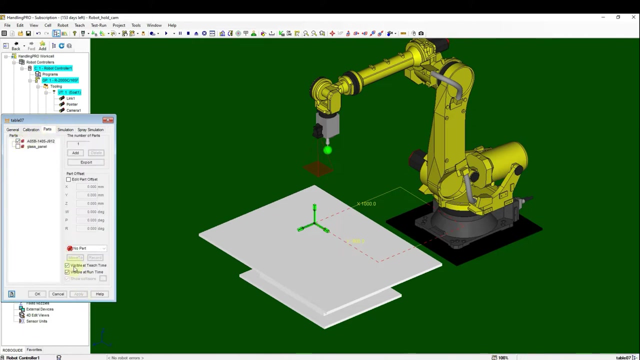 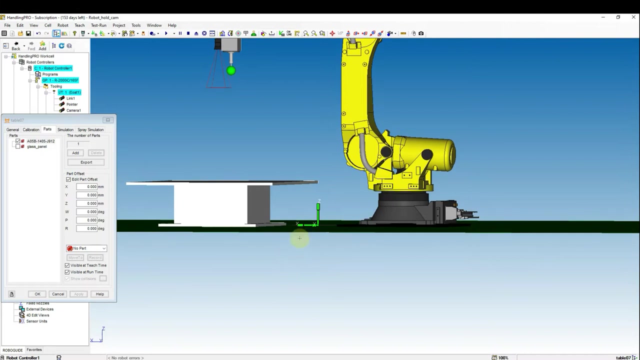 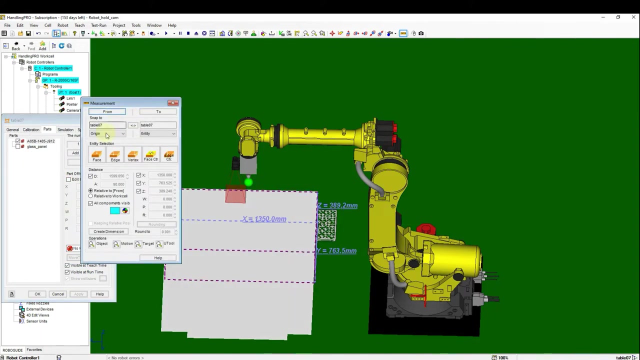 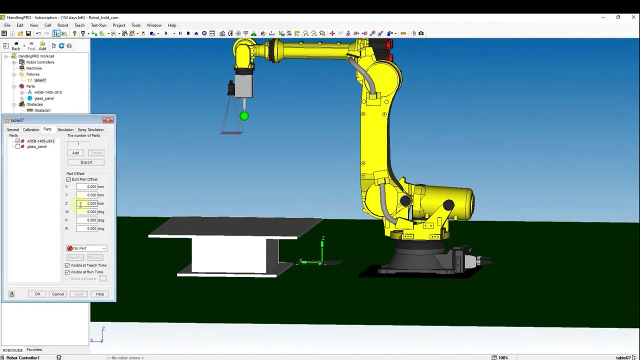 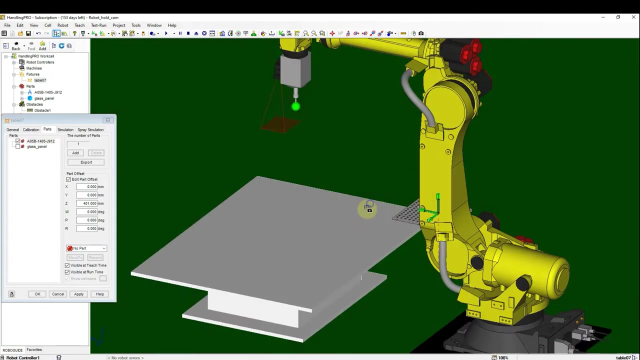 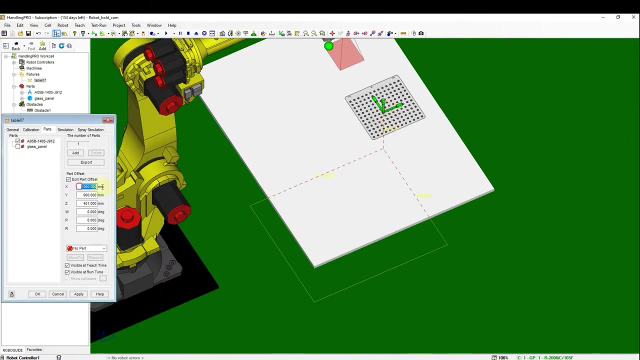 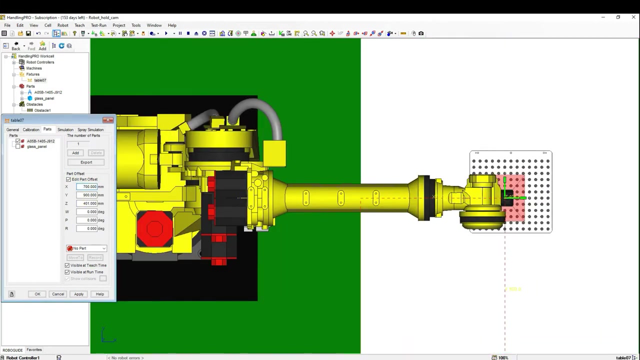 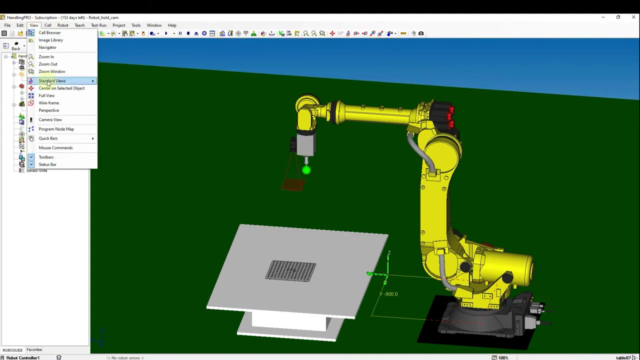 Set the size accordingly. Double-click at the table and then select Part tab to add part. First set the calibration jig to slightly higher than the table top, Then move it to robot camera view center. We can check the camera view with the view menu bar and then select camera view. 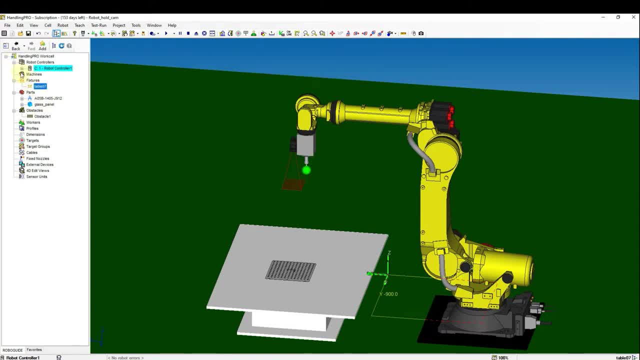 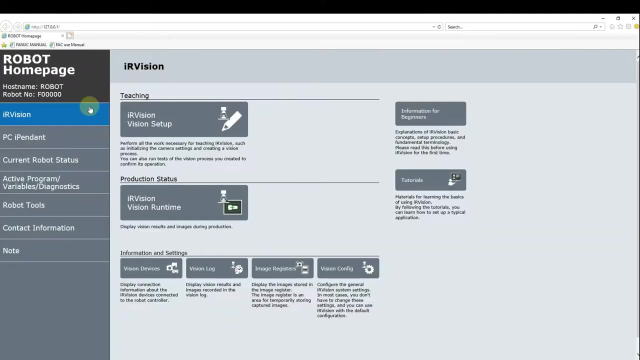 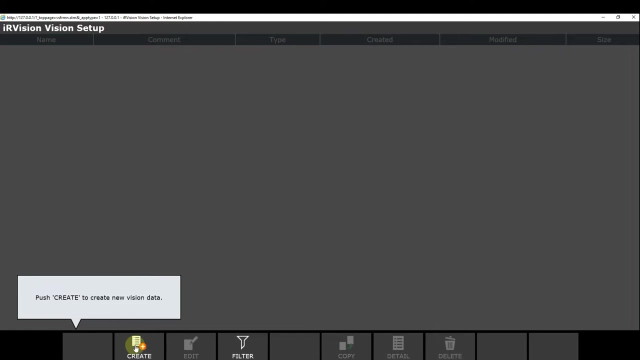 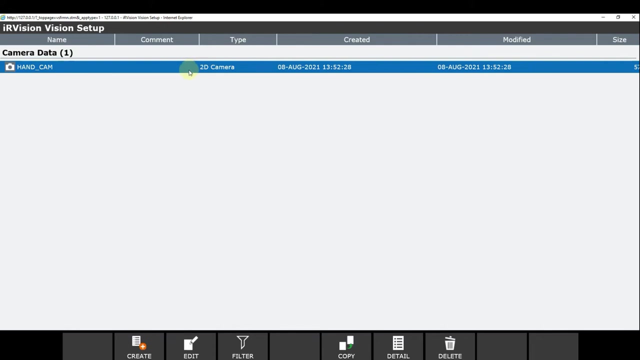 Now go to the cell browser and then select the vision menu With the general tab, click the, the port 1 and then select device to map to it. From the top menu bar, select robots menu and then select internet explore option, Click the, the vision setup button and then create the camera data. 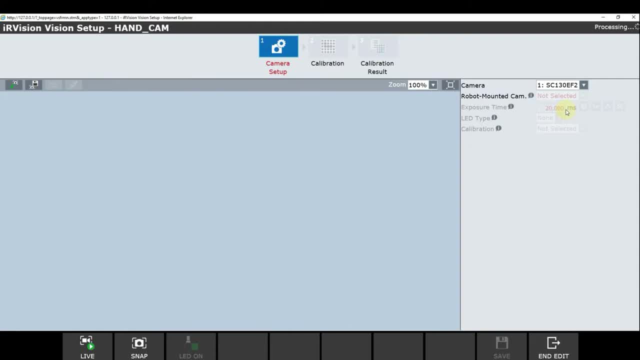 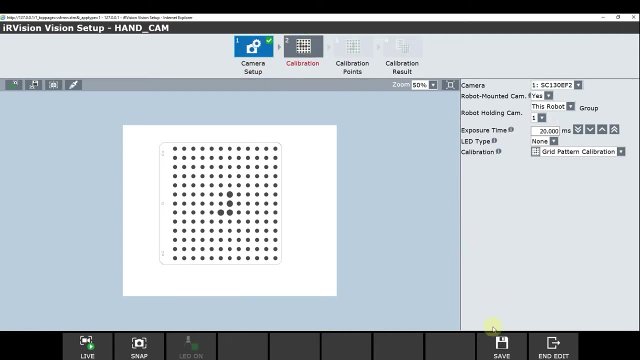 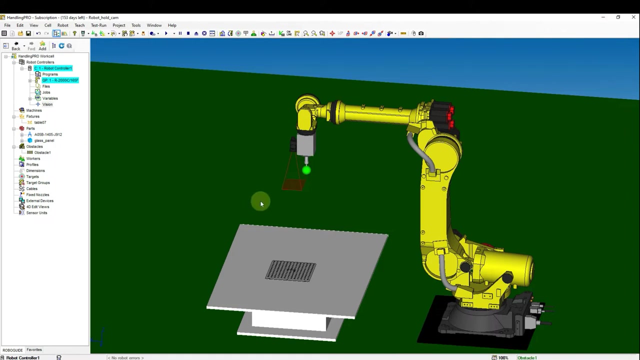 Set the camera and then select the camera view. Then choose yes for robot mounted camera option. Then change the calibration option method to grid pattern calibration Temporary. save the data Now. move back to the robot guide screen. Now open the camera view. 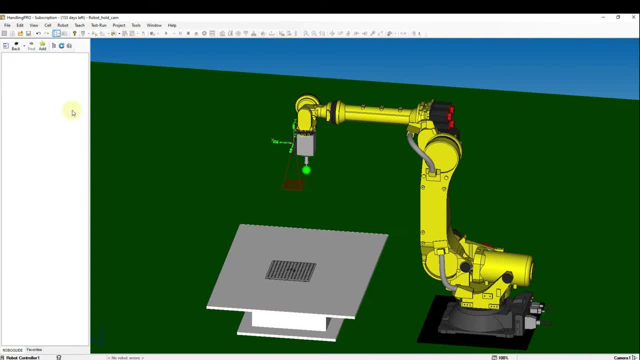 Select camera properties from the UT1 and then select the setting tab. I do like to change the focal distance to 16 mm for more detail image. After that go to view tab and change size to 1250 mm and then visible setting to only when snap is done. 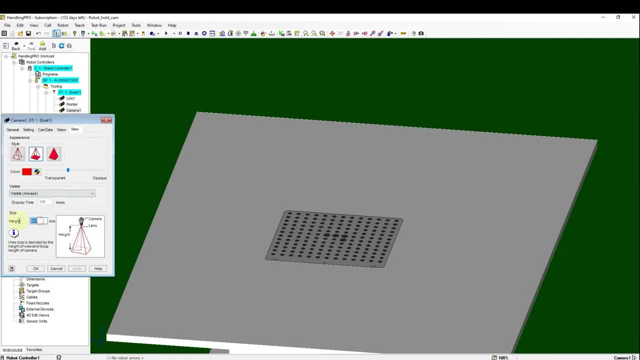 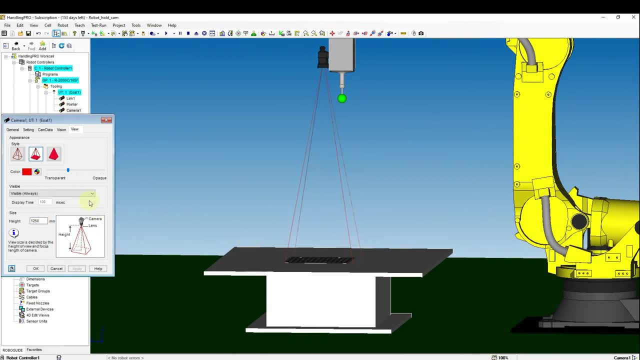 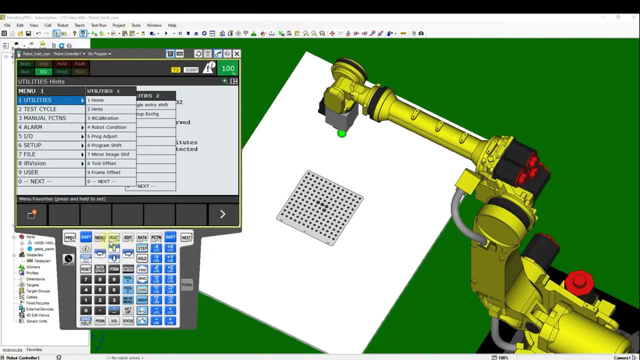 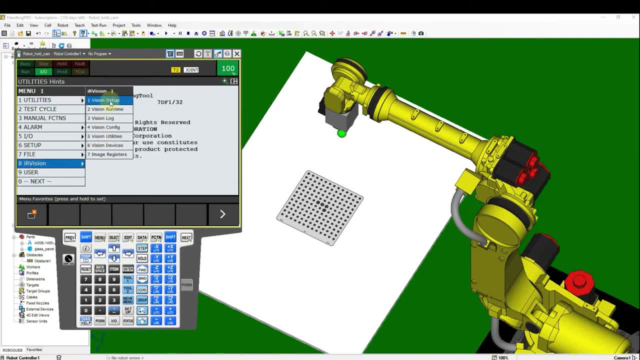 Then select IR Vision Utility. Select IR Vision: Hational Photography答案 nuestros. The priority screen shows the settings for touch screen and then SELECT IR Vision Utility. From the utility screen, choose the automatic grid frameset, Then select 안τη câc. 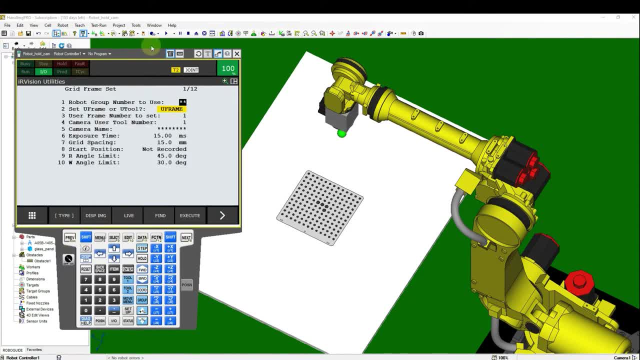 grid frame set. Set the group number as 1, and then remain the user frame and user tool number. as we are using the empty frame. Change the camera name to the camera we connected to robot earlier. After that, change the grid spacing value. 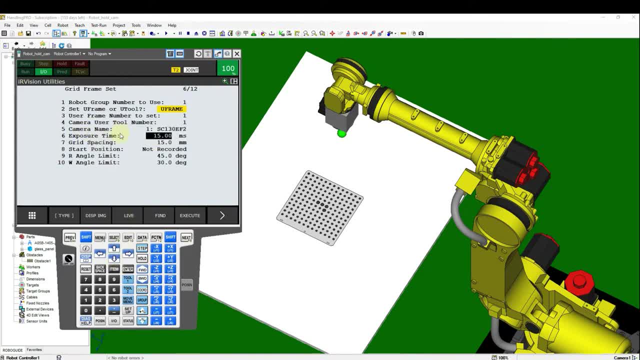 to 30 millimeters. Record the current position as start position. If we need to confirm the current recorded position can fully view the calibration jig: click the display image button on teach pendant screen and click find button to check the image result. After confirm all settings, move away. cursor from start position setting. 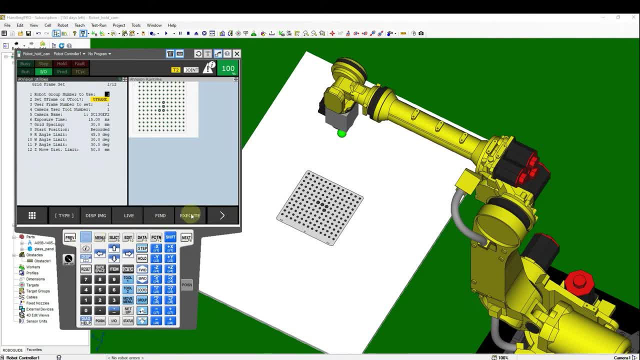 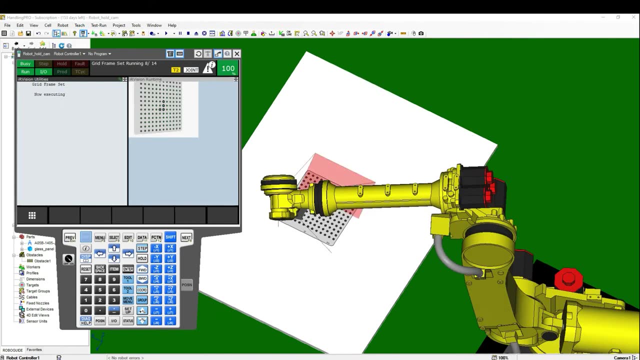 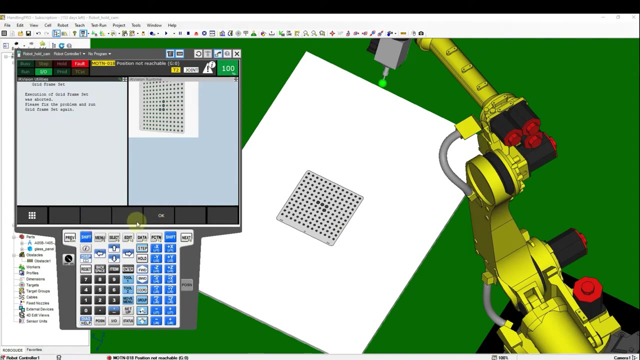 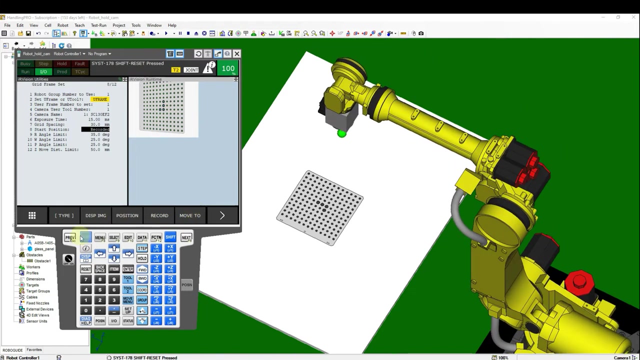 hold down shift button and then click execute button. If we found the alarm as position not reachable or axis limit, we need to reduce the WPR angle limit, Reset the alarm and move robot back to start position. then execute again When dialog showed select restart to continue. 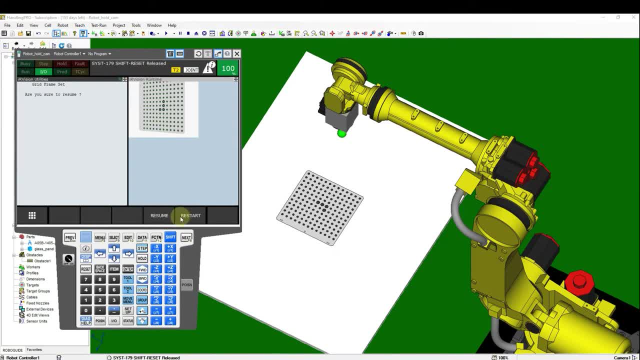 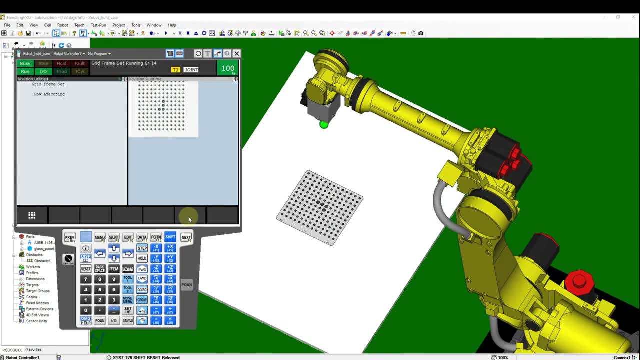 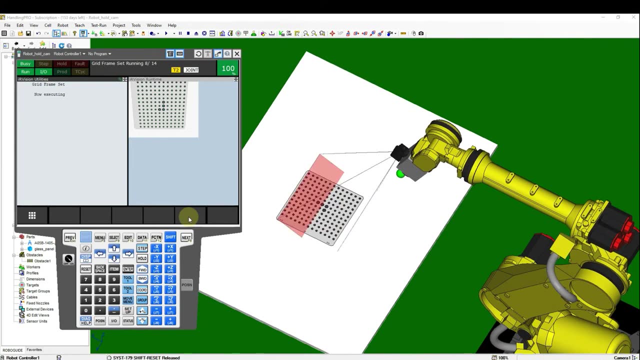 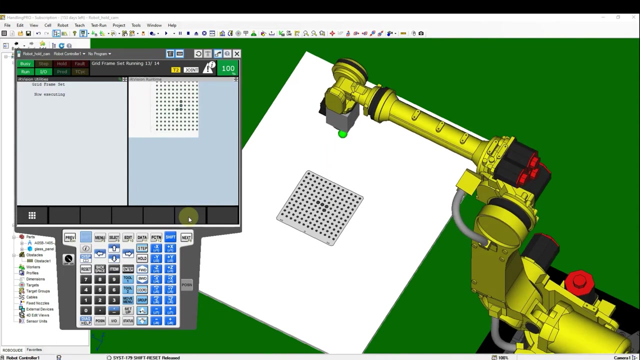 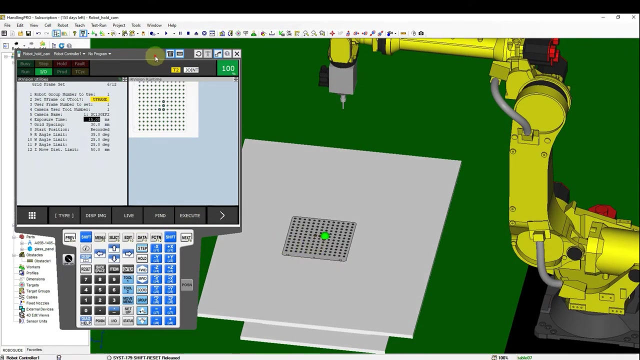 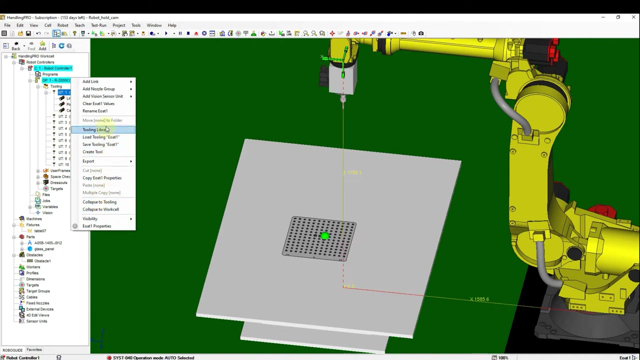 Robot will move for 14 procedures to confirm the center point of calibration, jig and camera center point. After completed of procedures, user frame and user tool data will overwrite by robot automatically. Now please copy UT1 setting and then paste at UT2, as we need UT2 to set the. 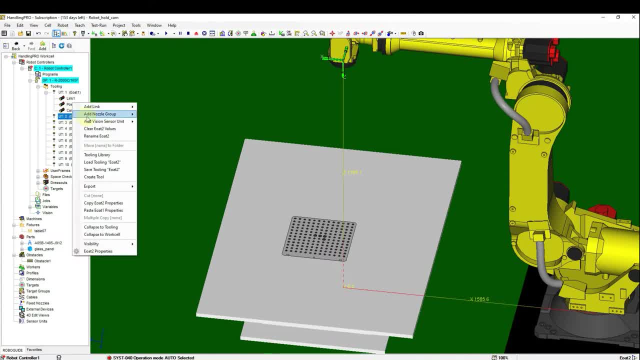 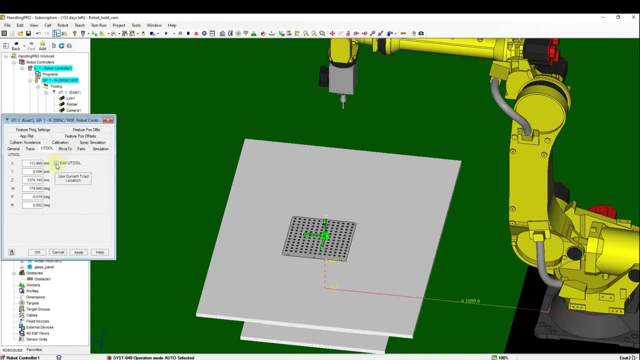 tool center point at sharp tip. Change the UT2 tool center point accordingly. Oaxqueyouorg, We hope you had fun video. it turns on sometimes and if you have data that we wouldn't be proposing, we found some. Can you use a little bit faster? 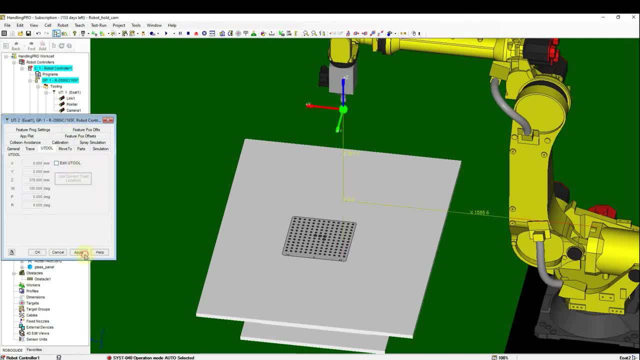 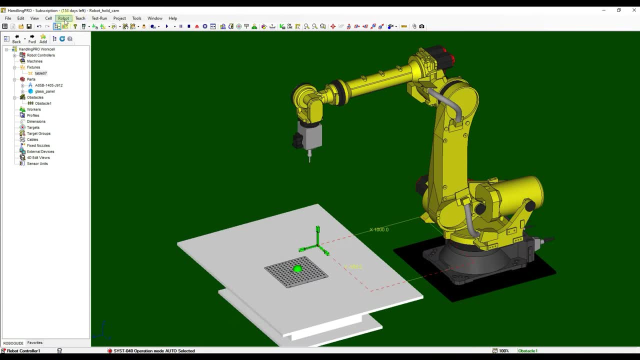 We did it, but it is sad. full speed. Now we create new upload, july 18.. Let's open the support appear back here. Please download online in the archive and upload now you Internet Explorer again and then click Edit button to enter the camera data. 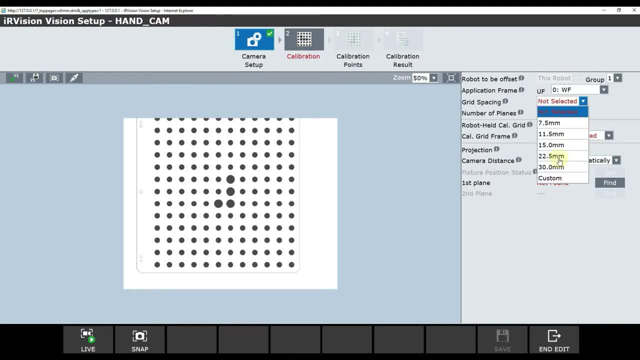 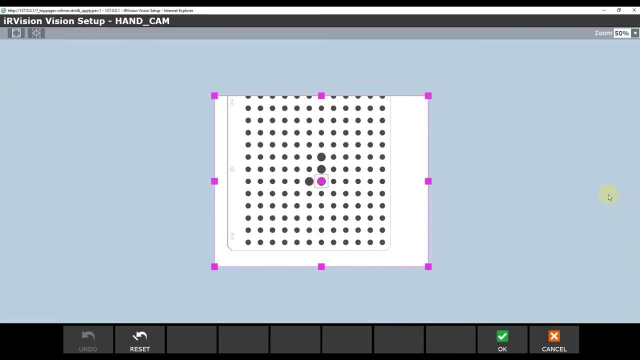 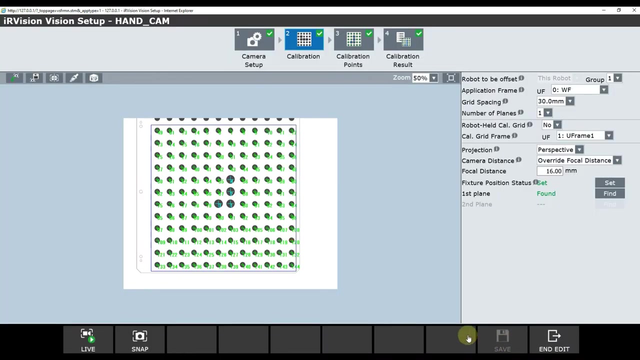 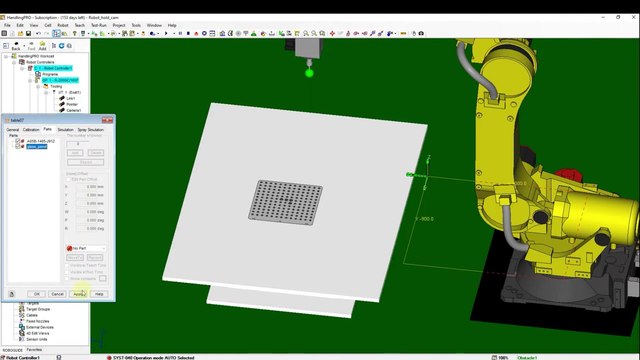 Go to Calibration tab and set the parameters accordingly. Move the square to cover as much as the full circle dot. Now our calibration was completed. don't forget to save it. We can check the calibration result at the Calibration Result tab. Now back to RoboGuide. add the glass panel to the table fixture. 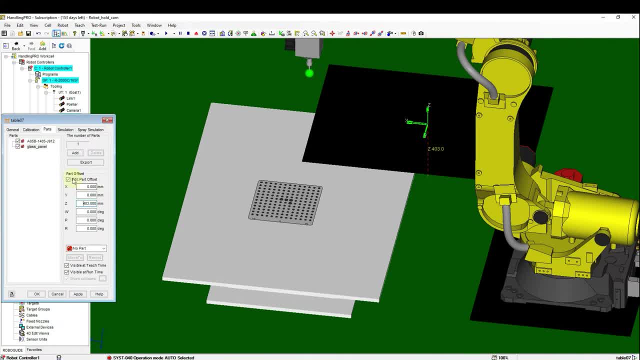 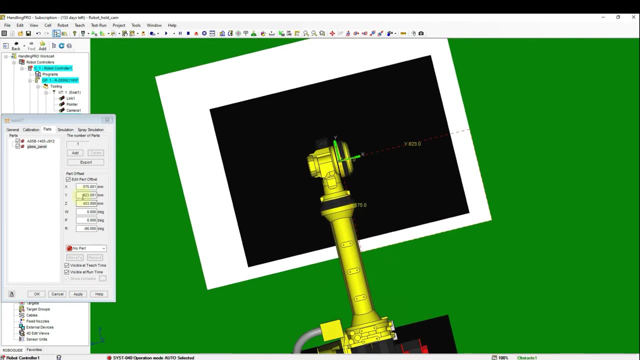 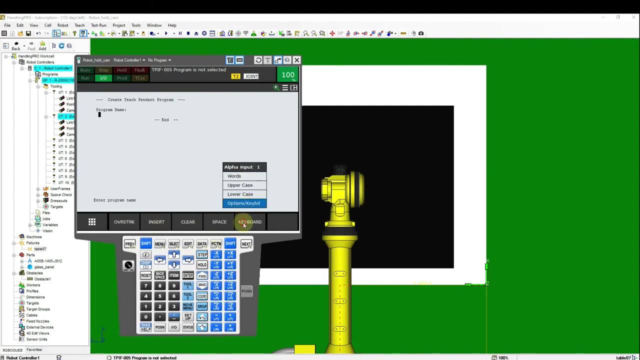 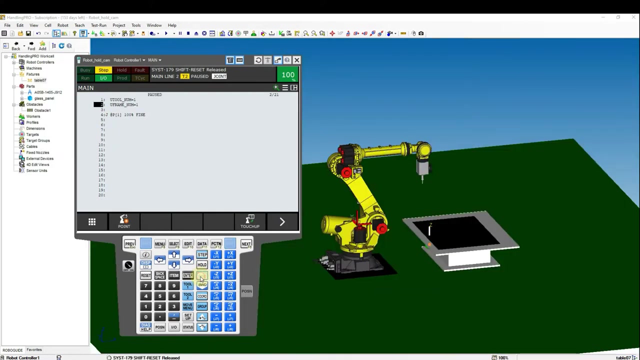 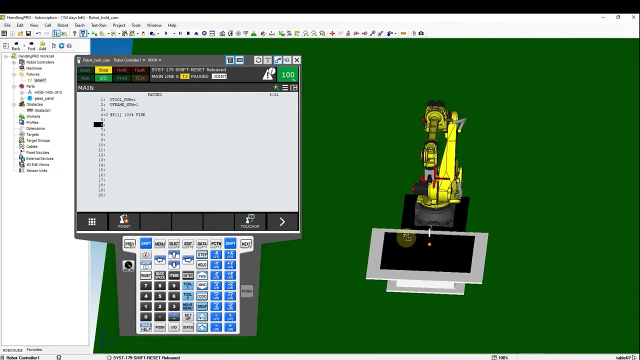 Set the location accordingly, Create a program and follow my step to add on the instruction. If you could not follow, Please have a view on my basic tutorial video. Thank you for watching. See you in the next video. Subtitles by the Amaraorg community. 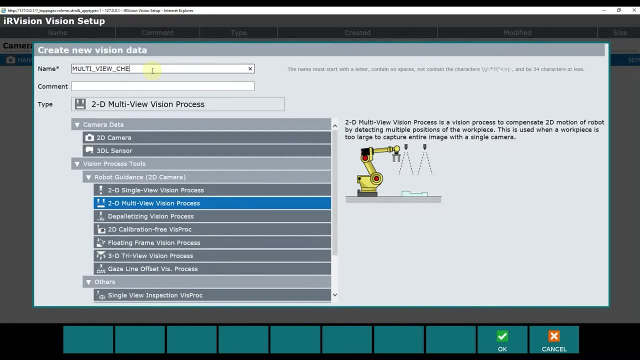 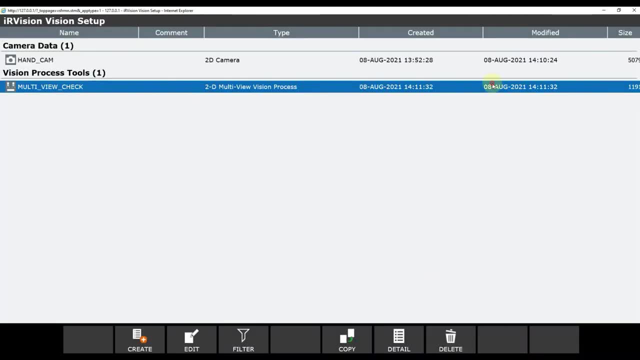 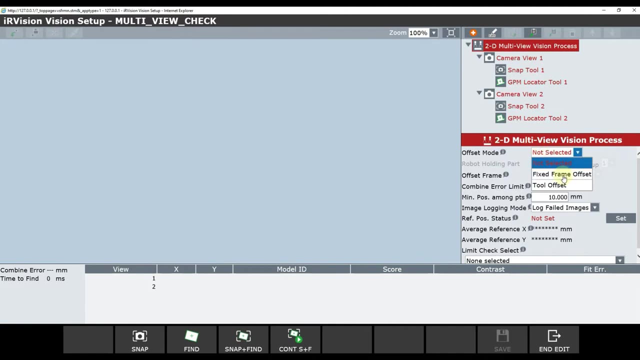 Subtitles by the Amaraorg community. At the 2D Multi-View Vision Process menu, set the Offset Mode and Offset Frame. Others item please remain and will set up later Subtitles by the Amaraorg community. Subtitles by the Amaraorg community. 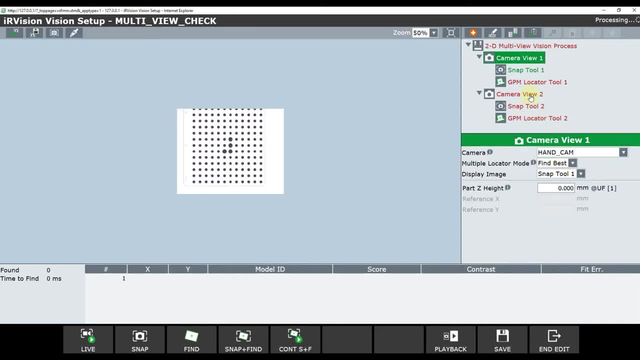 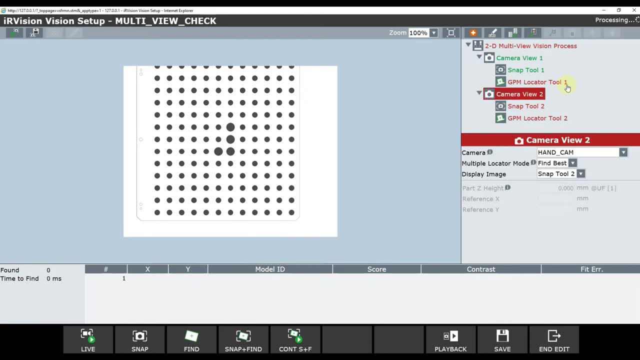 Subtitles by the Amaraorg community. Click on Camera View-1 and set the camera data we created and calibrated just now. Repeat the same thing to Camera View 2 and 3.. Move selector cursor to 2D Multiview Vision Process Menu. 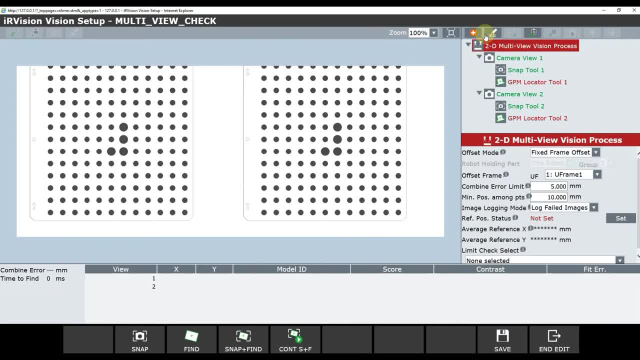 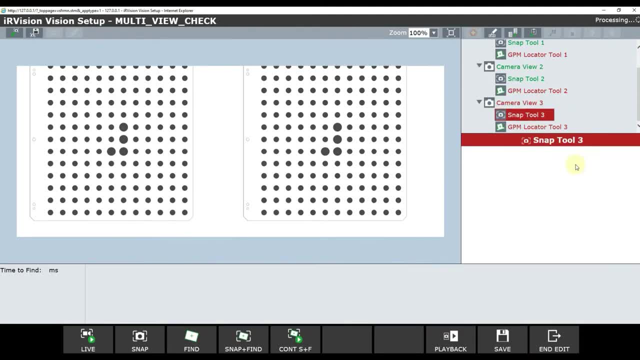 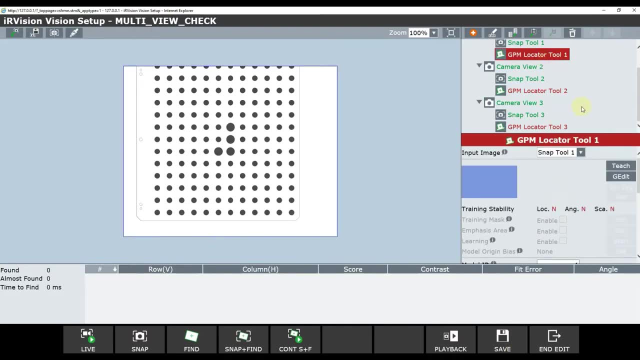 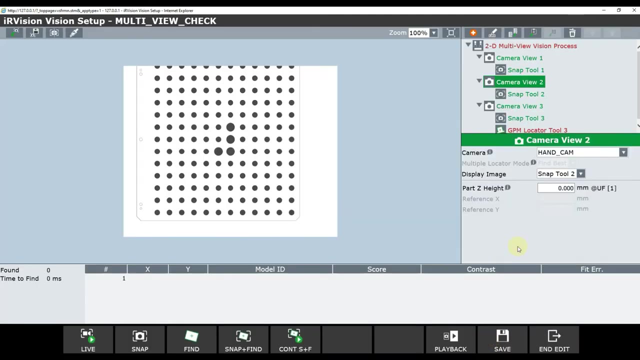 and then click add button and then add Camera View 3. Default Vision Process Menu, κάνpas a tab key shortcut. vision process for camera view is using GPM locator tool, but our workpiece is not suitable to use this tool. please delete all camera view GPM locator tool. 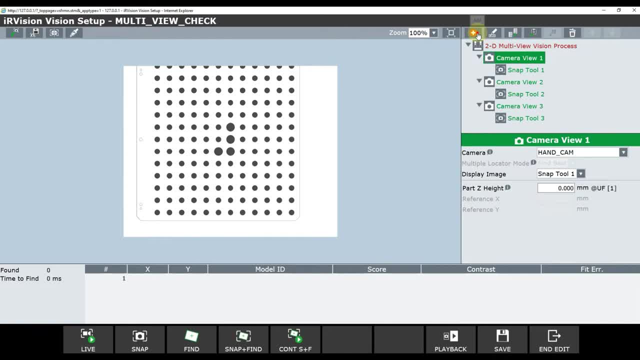 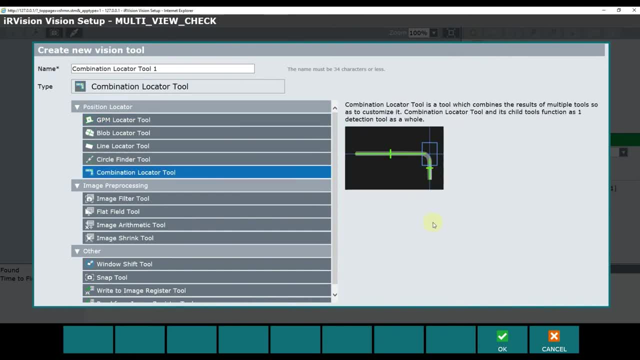 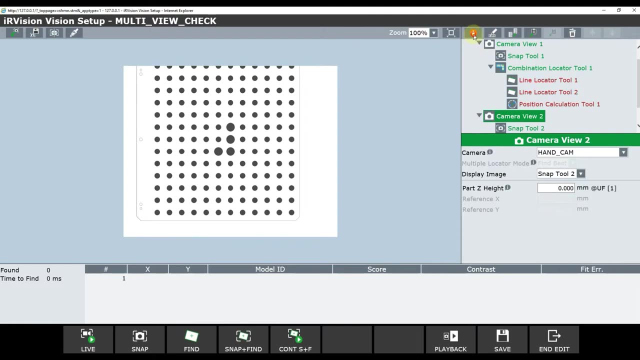 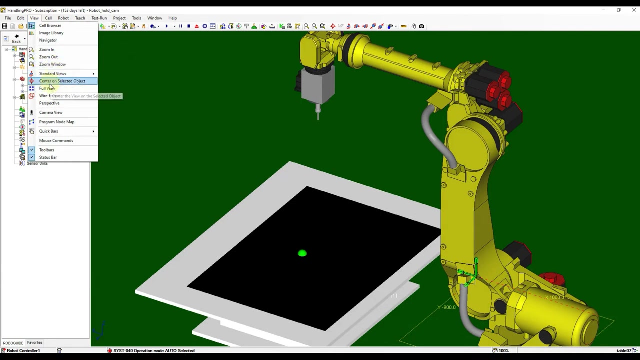 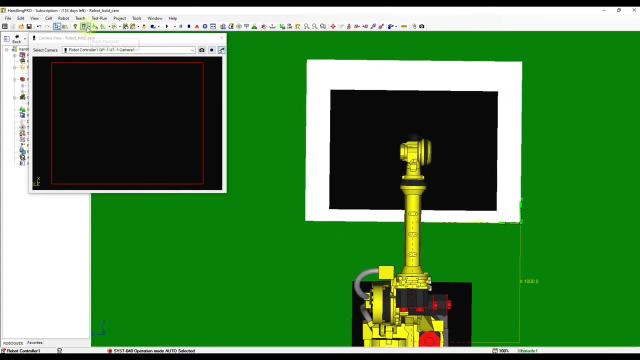 now select the camera view one and then click Add button. select combination locator tool from the list and then click OK. repeat this step for camera view two and three. you back to Robo guide screen. go to view menu at top menu bar and select camera view from the list. switch to top view of work cell. then. 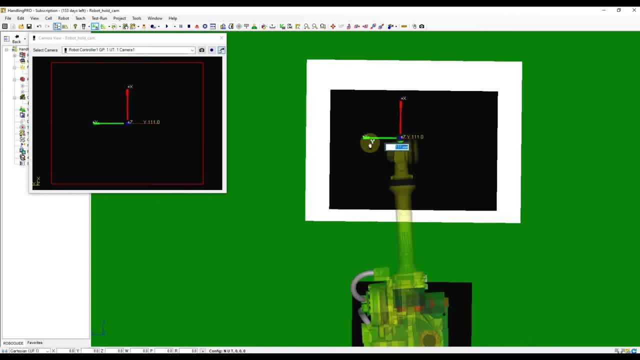 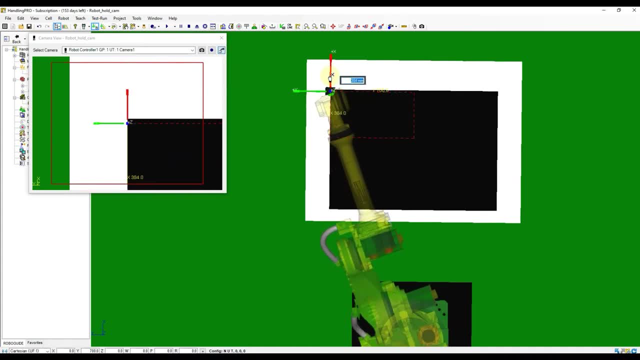 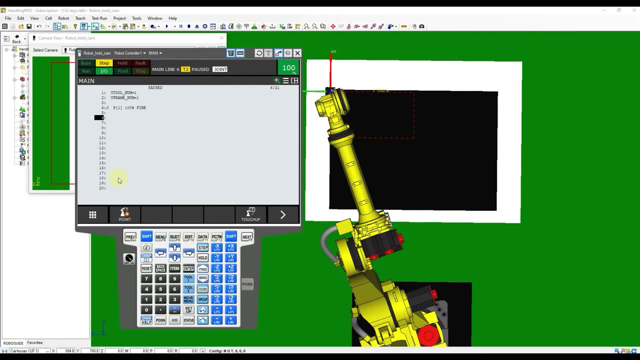 click at the teach tool selection button to show the jog trial. I add, move the triad to the top left corner of the work pieces. after that turn on the teach pendant and confirm the user tool number and user frame number are in correct number and then record the first snap position in. 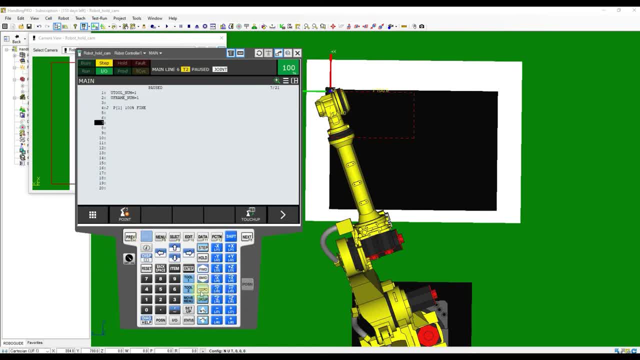 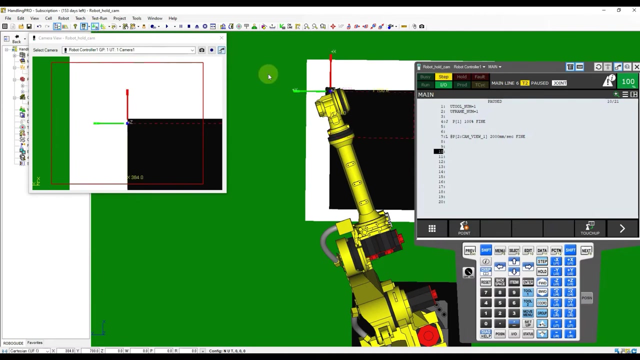 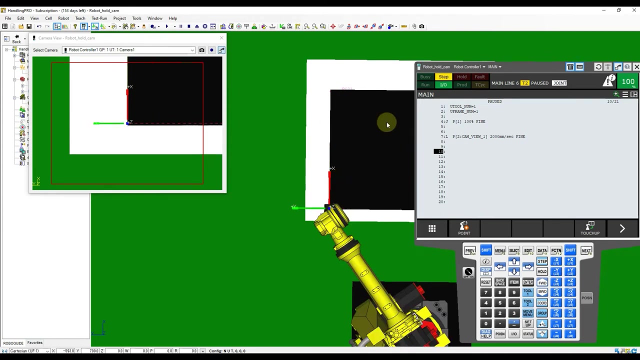 the program we created just now. repeat this step to bottom left corner and bottom right corner of the work piece. repeat this step to bottom left corner and bottom right corner of the work piece. so for both degrees the acceptance value is 0 to 0. please make sure you make some reserve lines at the bottom of the snapping points. 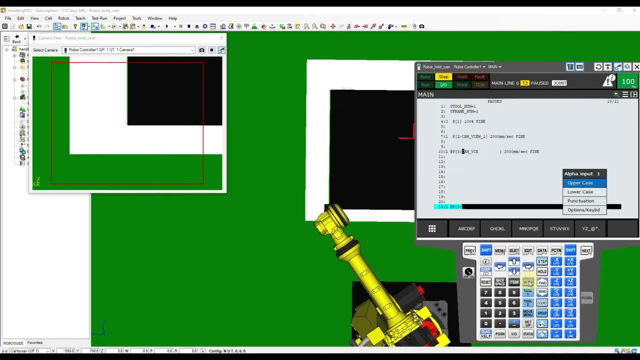 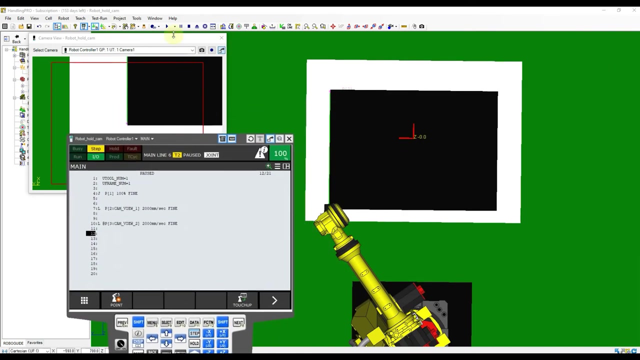 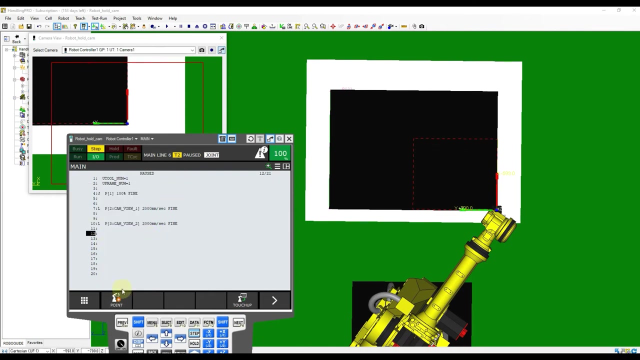 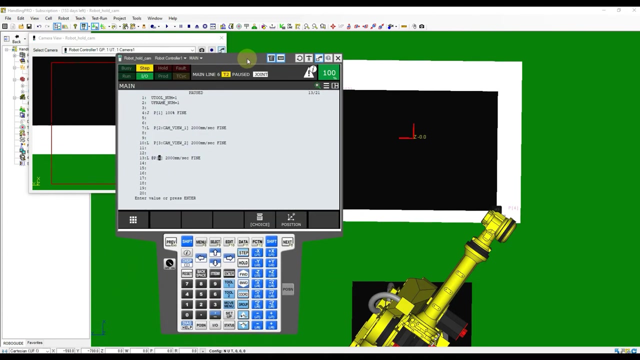 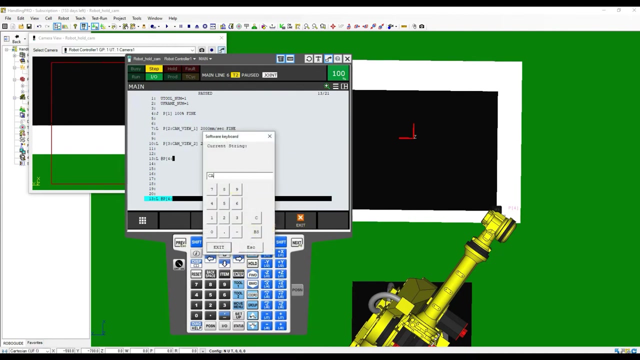 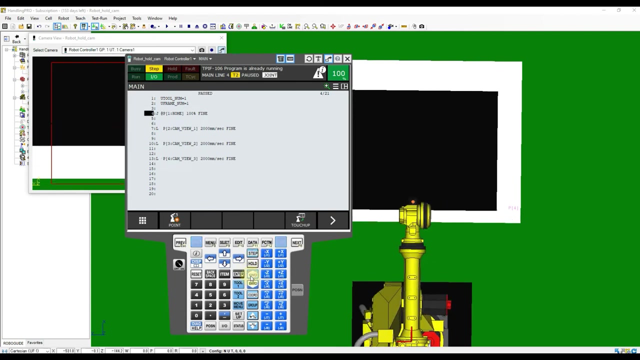 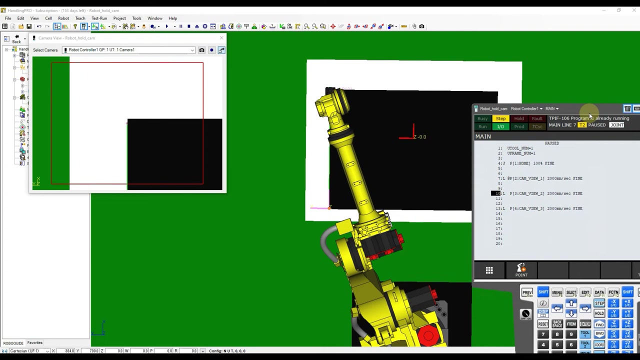 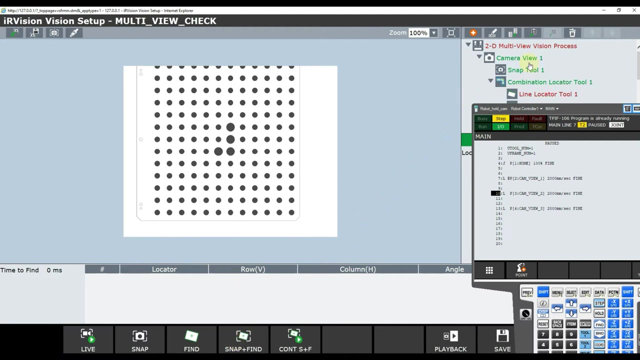 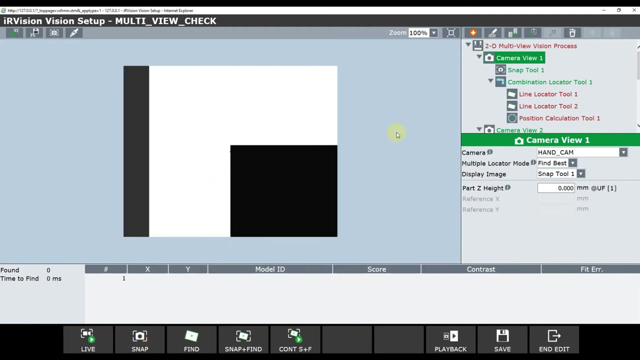 you, you, you. After completed the position touch-up, move the robot to with the program to first snapping point. Open the Internet Explorer again and then select the camera view 1.. Click the Snap button to update. Select the image, Then select the line locator tool 1.. 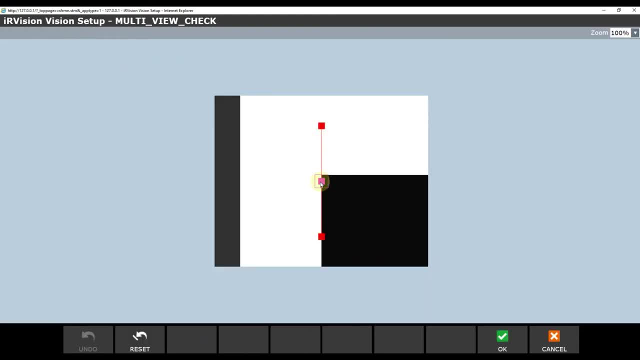 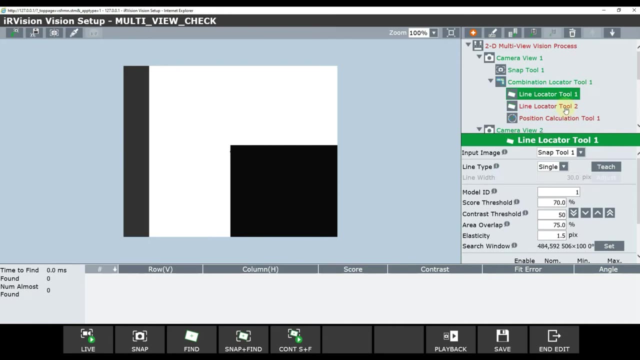 Click the Teach button at the list below. Drag the line to one of the edge of the workpiece and align it nicely. Click OK to complete the teaching and continue. select line locator tool 2. Drag the line to another. Drag the line to the other edge of the workpiece image and then click OK. 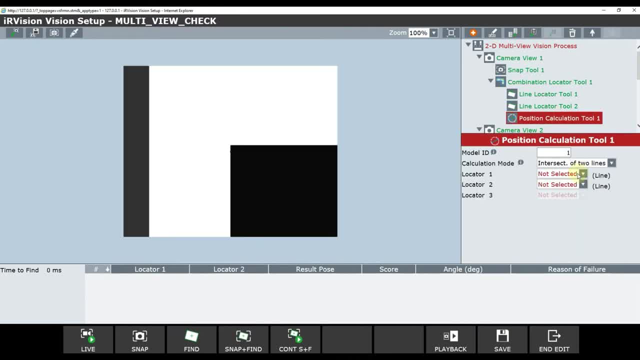 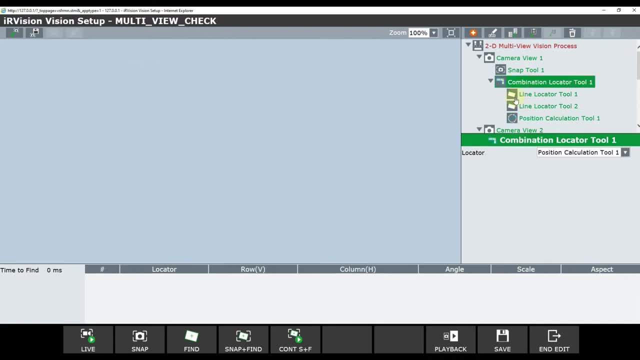 Now click at the position calculation tool 1.. Set the locator 1 and locator 2 to the line locator tool number. After that click at the combination tool 1 and then click Snap plus Find button to verify the teaching. After complete view 1, select camera view 2.. 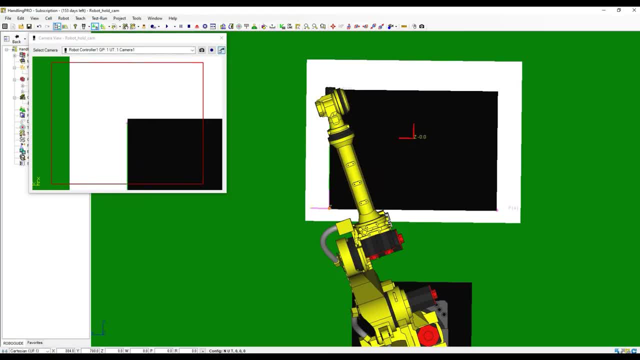 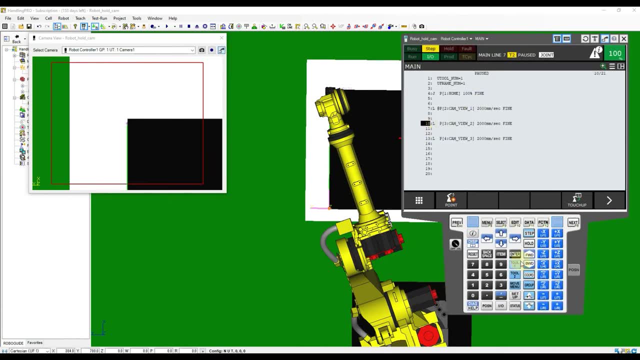 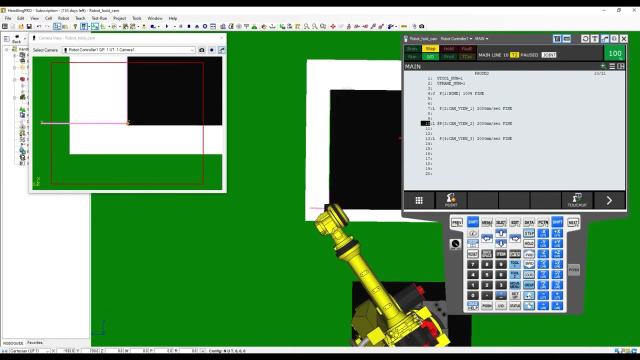 Back to RoboGuide. open Teach Pendant again and move to the second snapping point. . . . . . . . . . . . . . . . . . . . . . . . . . . . . . . . . . . . . . . . . . . . . . . . . . . . 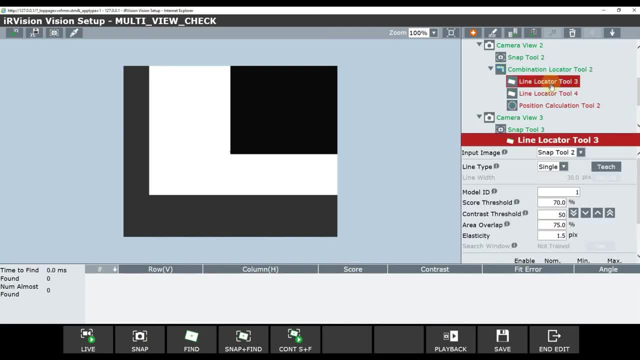 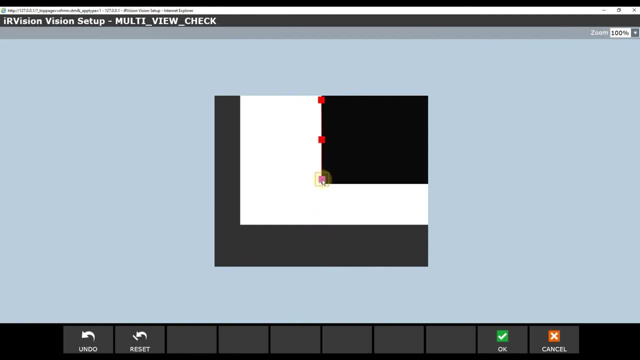 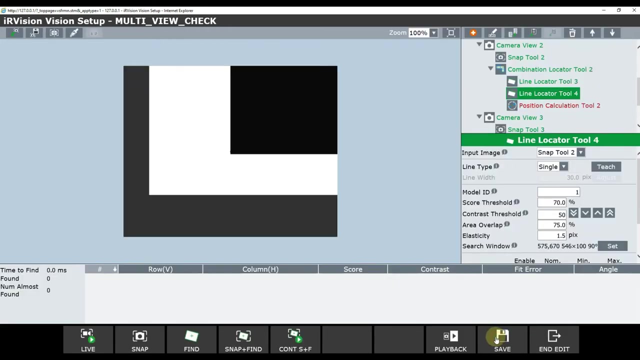 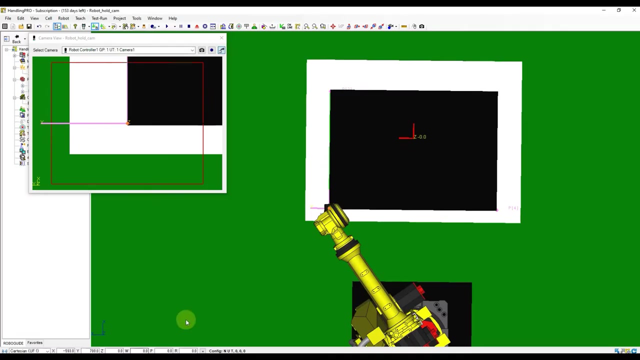 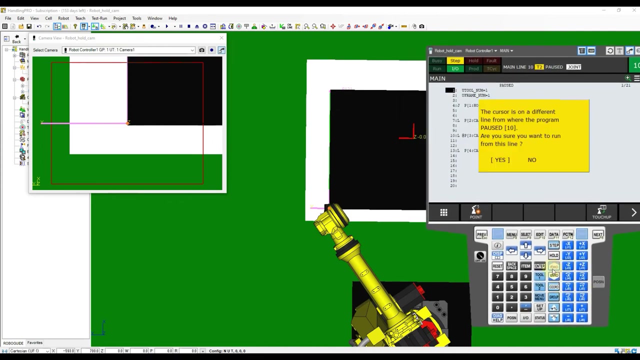 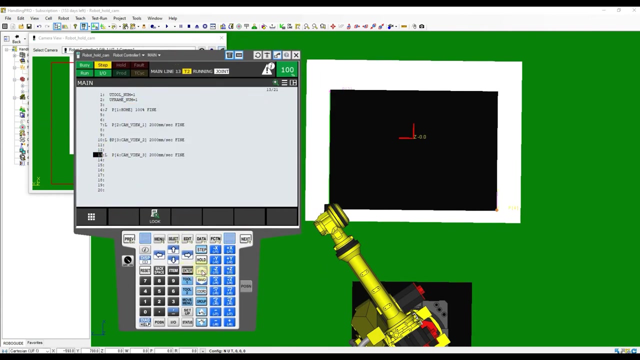 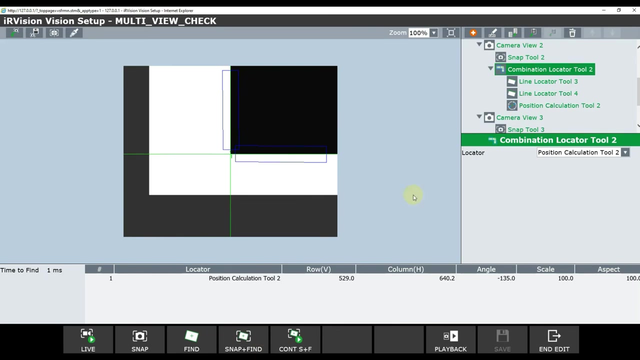 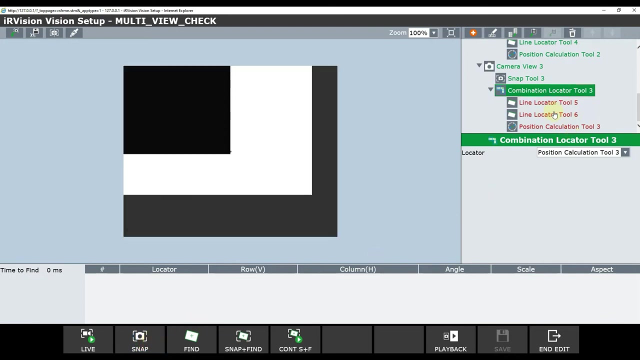 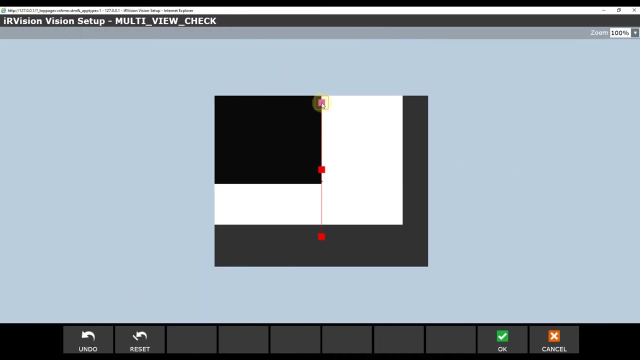 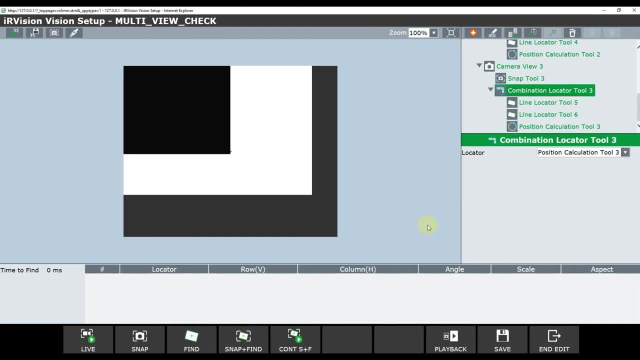 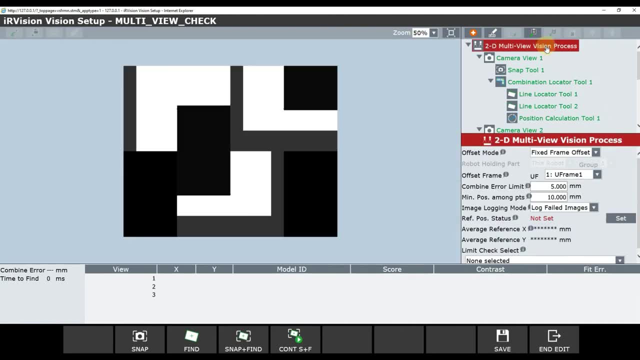 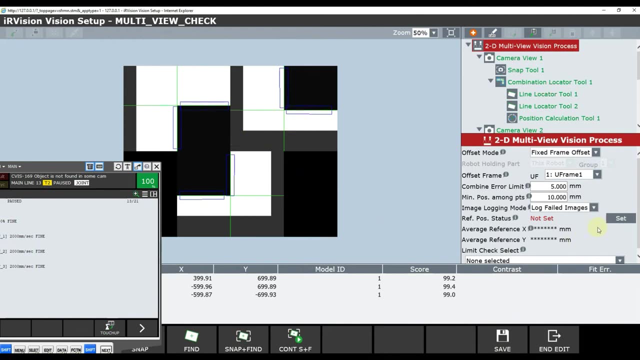 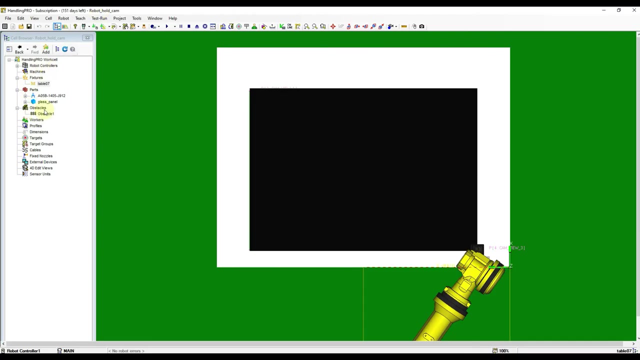 After completed all locator tool teaching, click at 2D multi-view vision process. Click Find button. if all three images showed on left, Find result success. click the Set button at the reference position status and then save the data Back to RoboGuide. 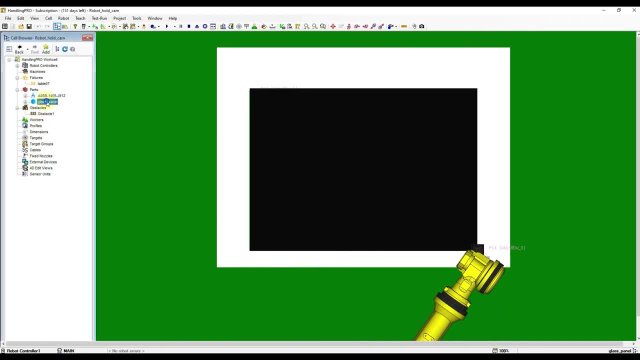 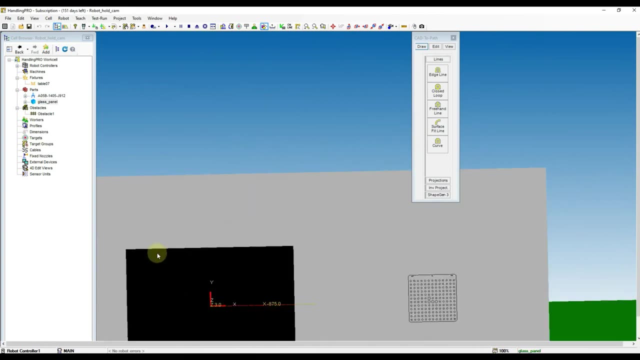 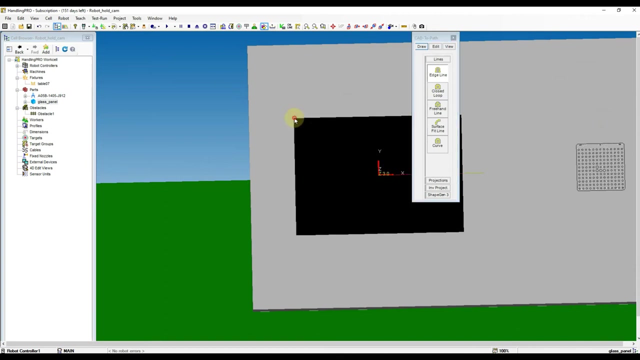 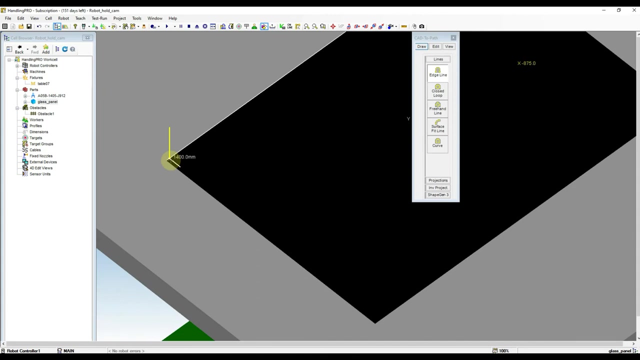 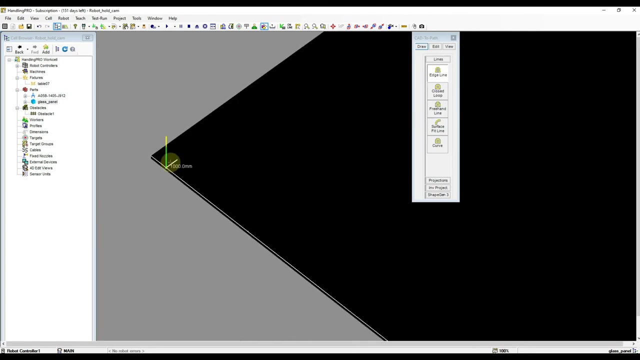 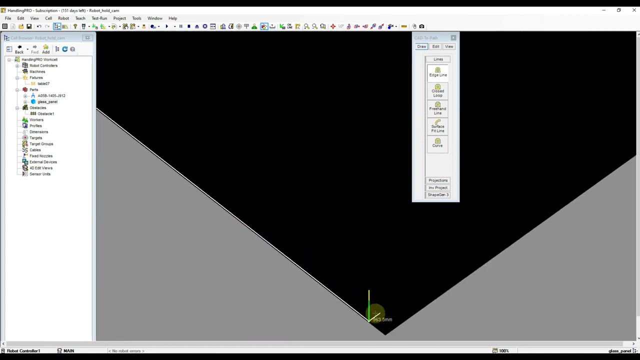 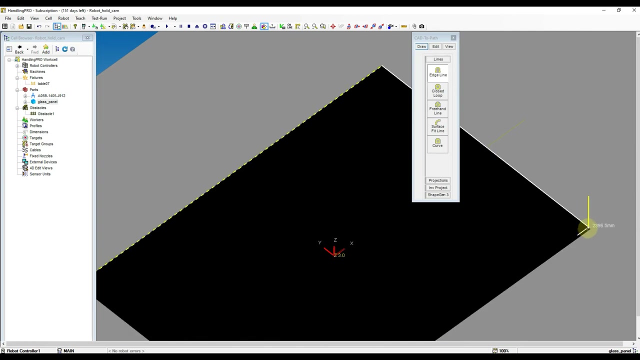 Go to Cell Browser menu and expand the Part menu. Right click at Glass panel and then select Draw feature option from the list. Click Headline from the pop-out toolbar and then start to plot the path on workpiece at partrack. Double click at the end of edge to complete the path plotting. 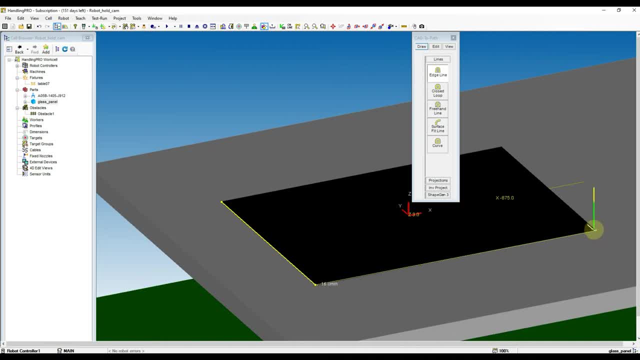 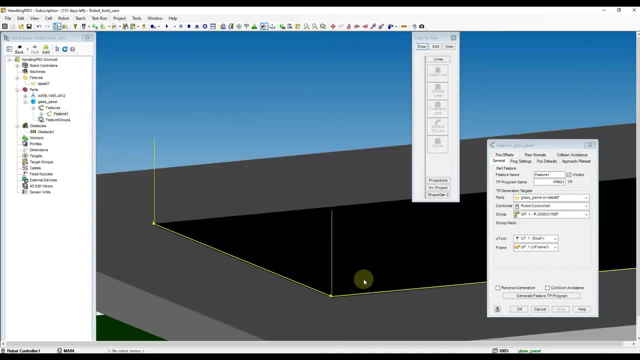 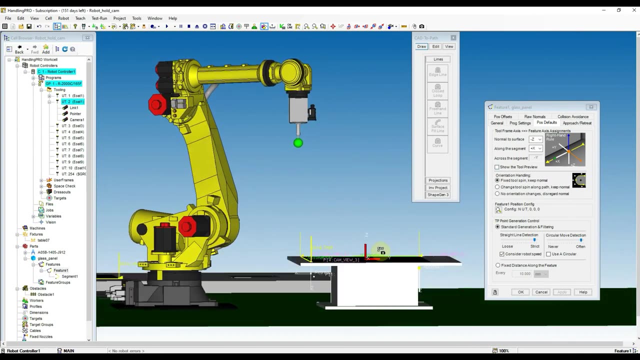 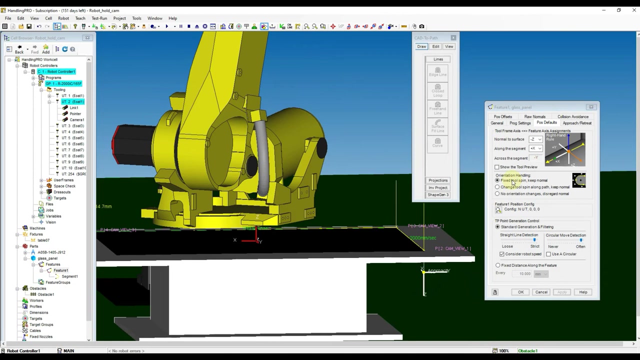 Confirm the path at the correct edge. Now move the view to the front of the table. We found that the orientation of triad created by the draw feature does not match to robot tool orientation. So please select Position Defaults tab and change the. 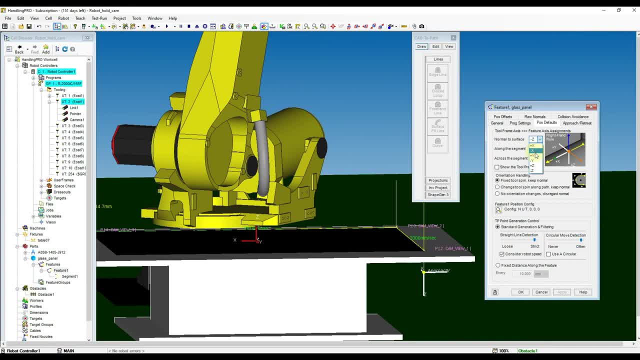 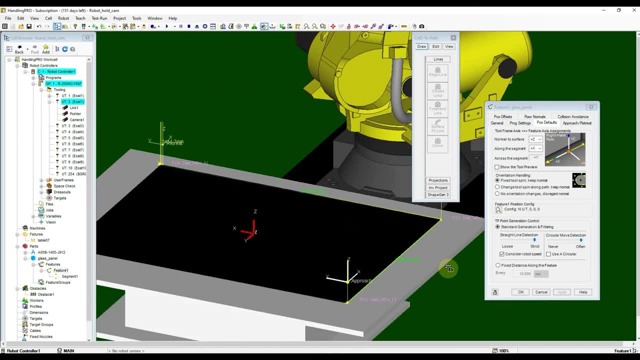 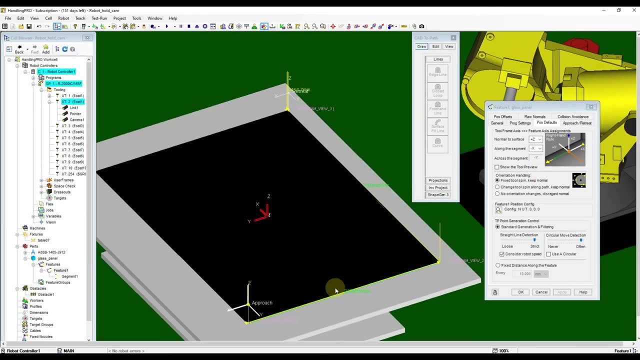 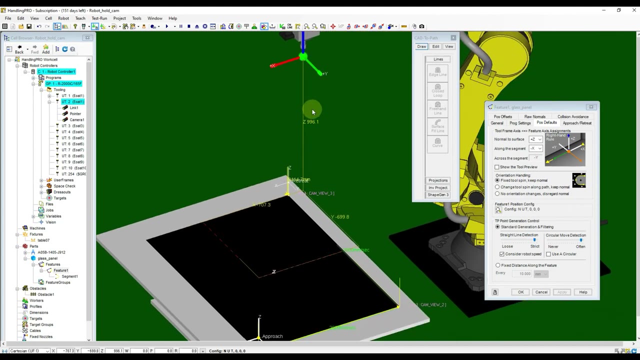 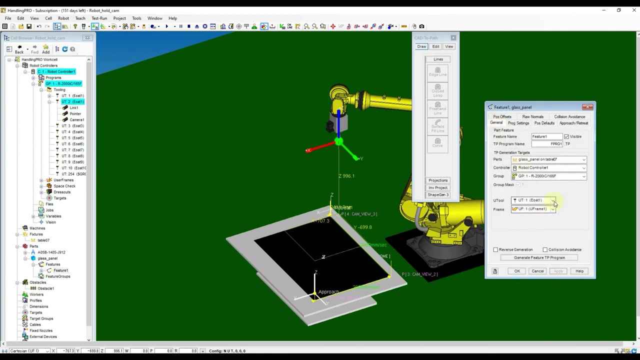 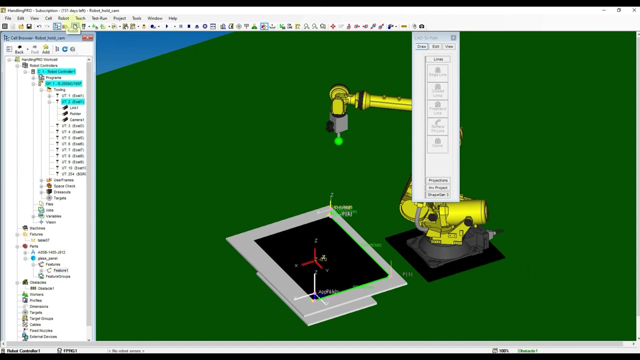 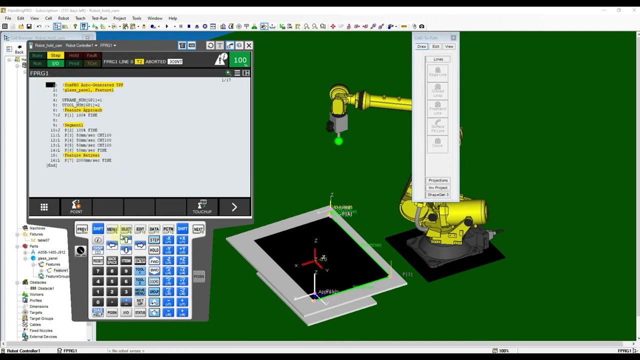 normal orientation. Now move the tool to surface and along the segment accordingly. Turn on the teach tool. selection of user tool. number 2 orientation. to reconfirm again: 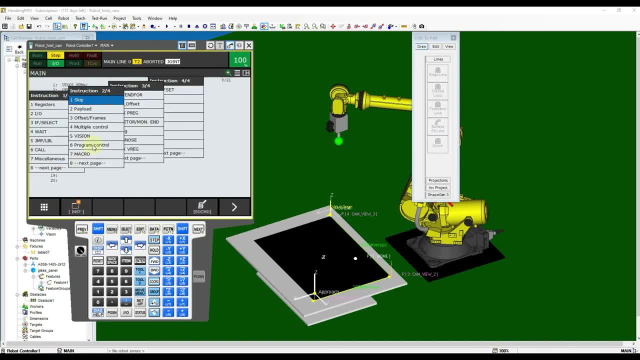 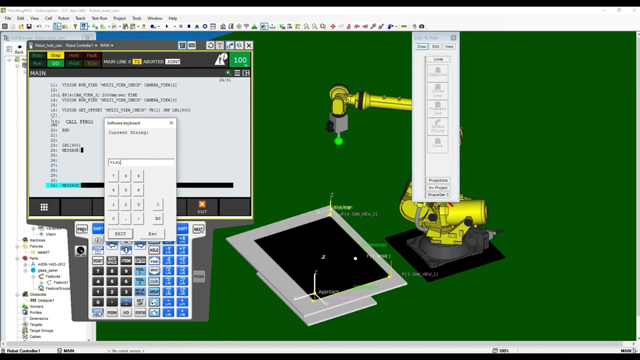 for each point. After done 3-point snap instruction. use Get Offset instruction to calculate the offset position of the latest image. Continue to input the program accordingly. Create the error branch label when the vision failed to detect the work pieces. Now the work piece is ready to be used for the next step. 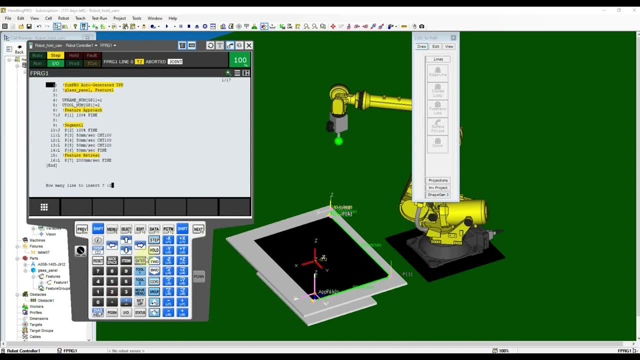 Now the work piece is ready to use. for the next step, We modify the generated program from RoboGuide, Insert the Vision Offset Condition instruction and then add additional motion instruction of Vision Offset at every single point. Now you can use the. 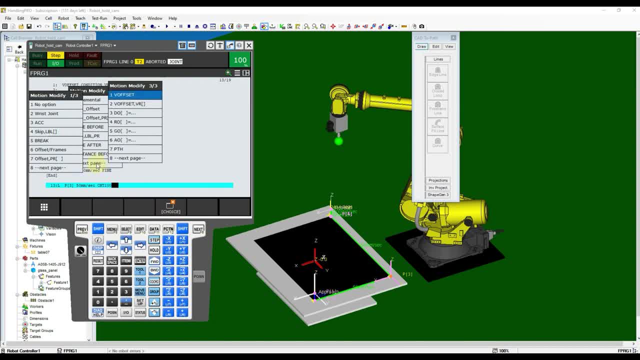 5th position to enter the work piece. The result is the same as the previous displayed function. Now we start adding the work piece to the work. To add up this work piece, click the button and then select the Mind on the work pieces. 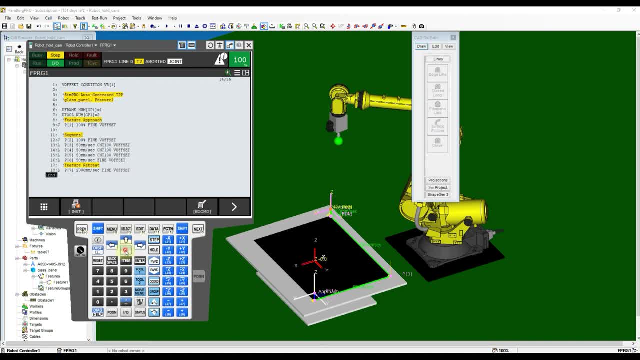 in the drop-down menu. The work piece will stop when you use the mind change. You can then stop the work piece and open the work piece. The work piece is now ready to be used as a work piece. Into the next step you will need to wanna start the work piece from the project base. 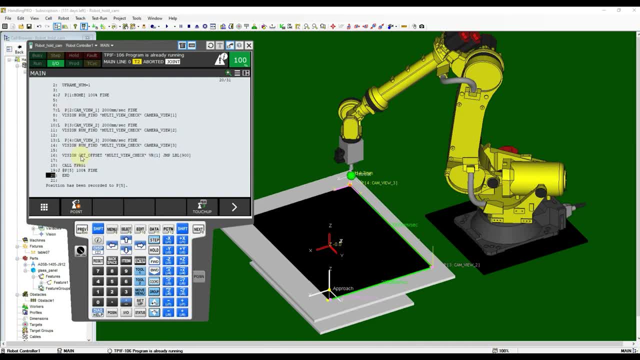 When you click on the work piece, click the button to select the work piece and then click the link to main program and then add the home position after the path motion. Remember to change the user tool number to 1, as home position is using user tool number 1.. 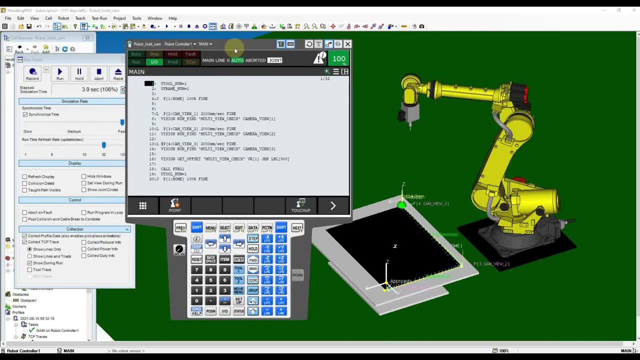 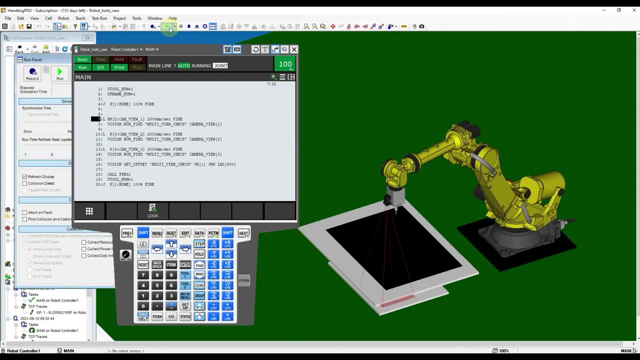 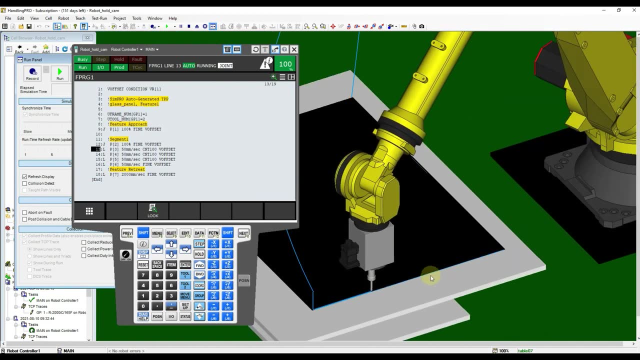 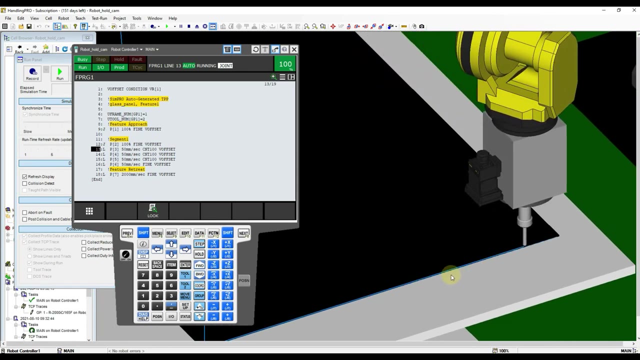 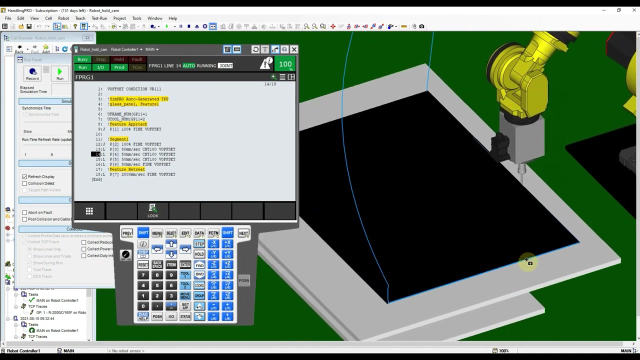 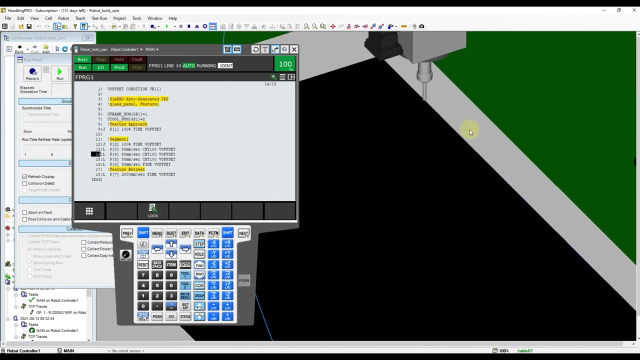 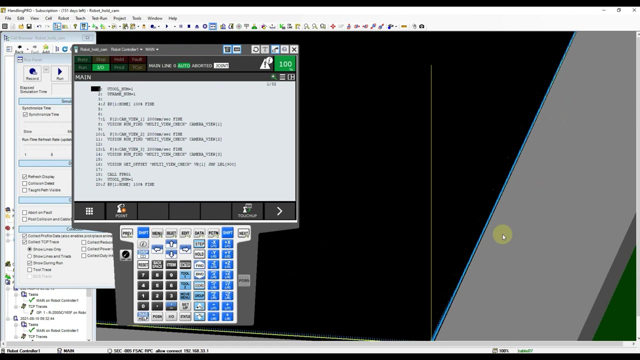 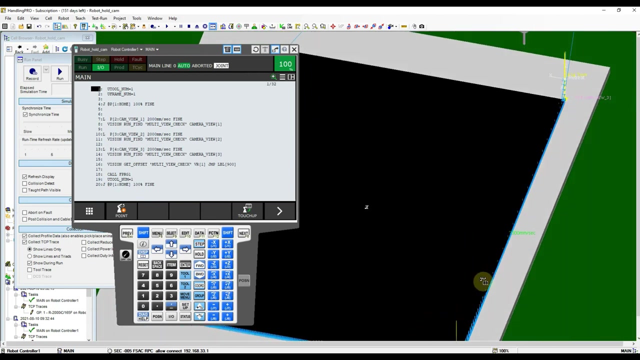 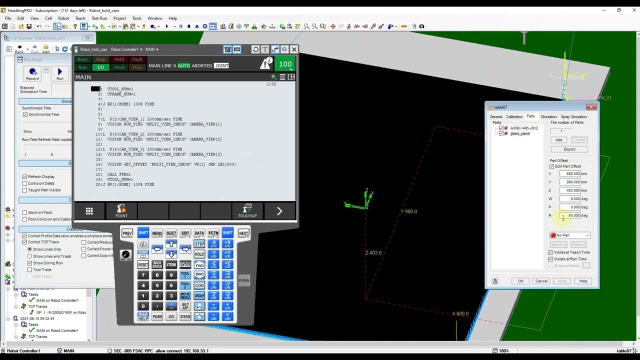 Now we can try out our program with click run button at top icon bar. After try out without offset the work pieces, now man will adjust the ROR value. Then test out the program again. Carefully monitor the TCP path lines. 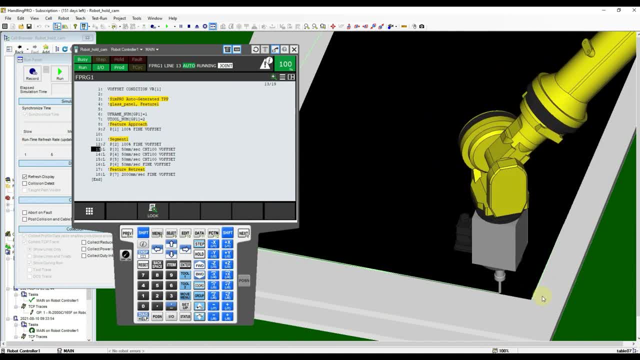 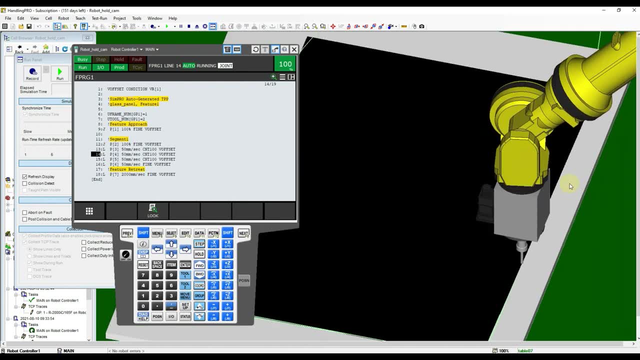 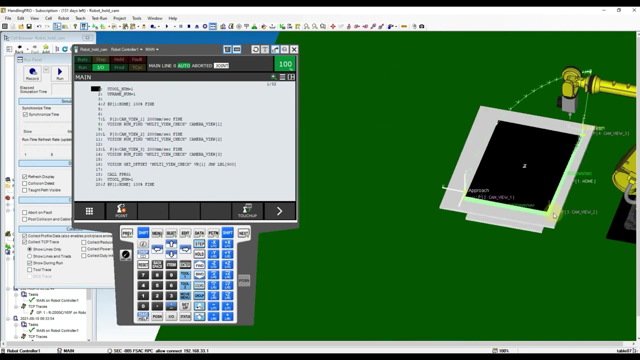 When you're done you can see the work piece has done. The process of working at TCP path lines is over. Now we can go back to our home page And try out the works-flow function. So here we can see the works-flow function has been convert. 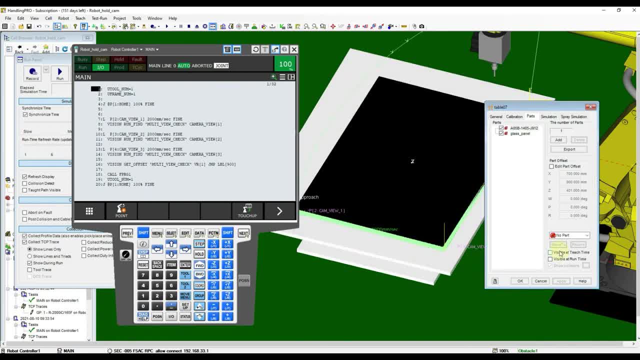 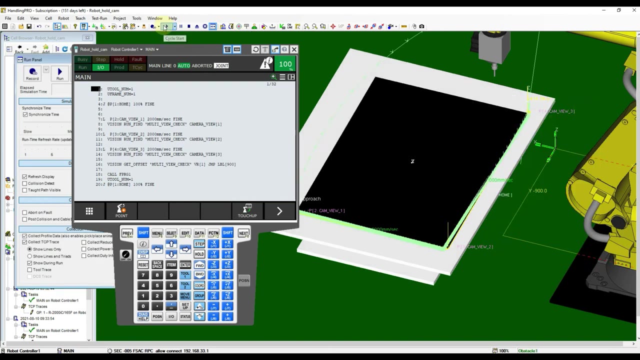 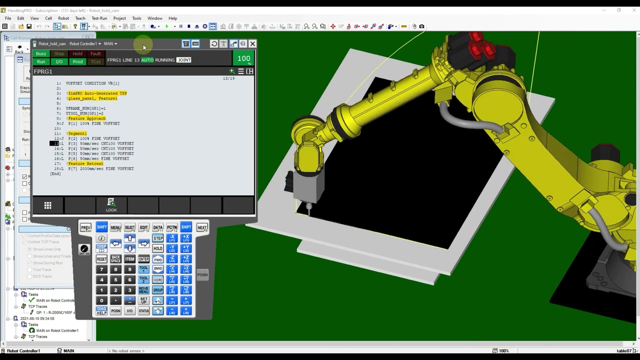 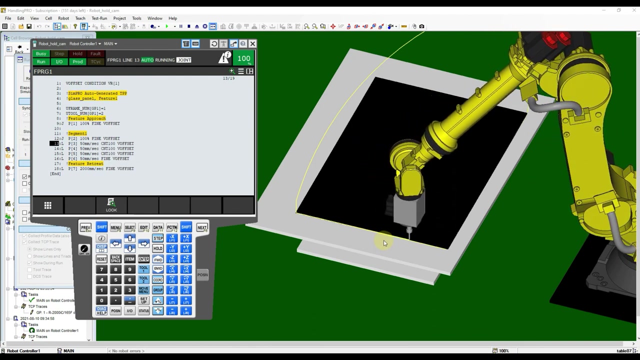 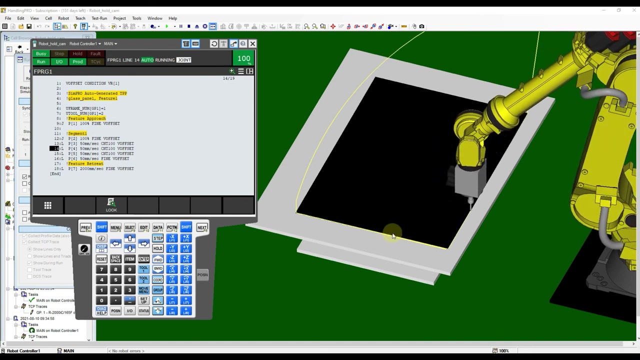 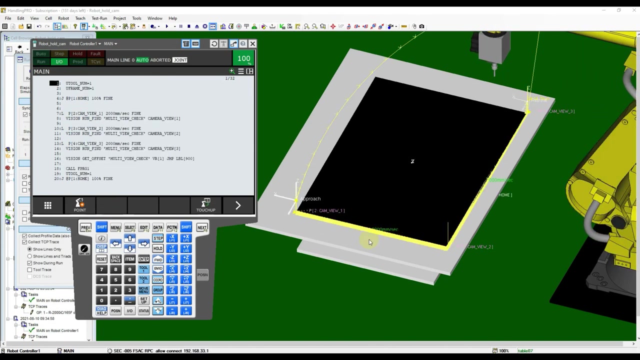 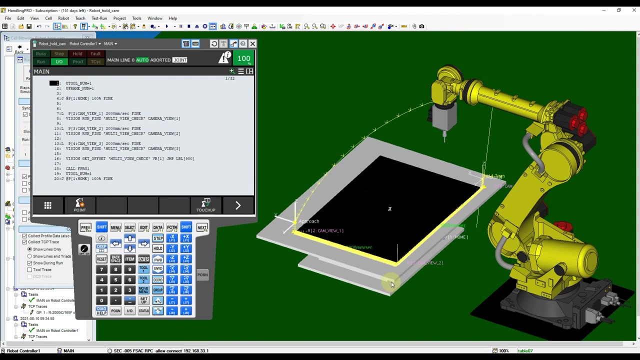 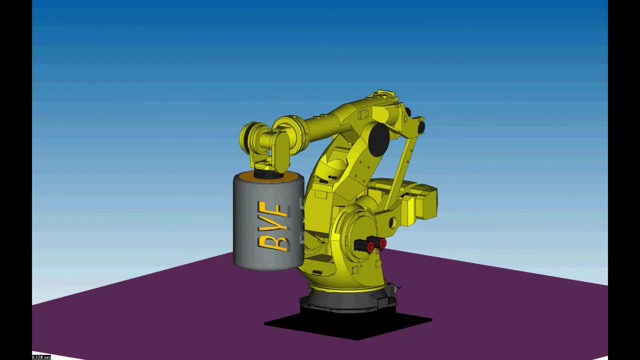 So that's the key point. I hope you use it. This kind of application is suitable for glue dispensing system and also edge deburring system. Please try your best to learn, Thank you. Thanks for watching and see you next time.